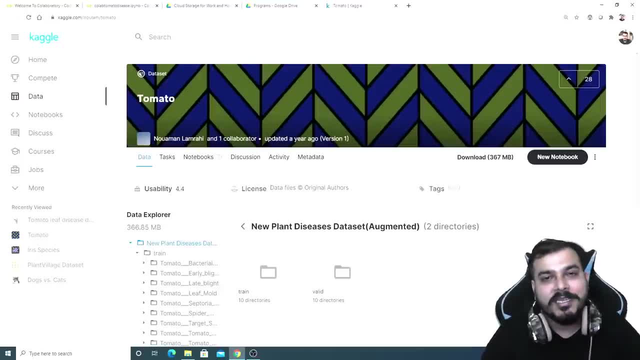 Hello, all my name is Krishnak and welcome to my YouTube channel. So, guys, today, in this particular video, I'm going to actually show you how you can train your deep learning models in Google Colab. Now, why I'm making this particular video, guys? because I see many people, you know they cannot just afford, you know GPUs and they cannot just use it for training. But Google Colab is a wonderful option. You can train any kind of things you know with respect to the data, with respect to the size of the data. If you have a huge data also, then also you'll be able to train. But, yes, you have to be a little bit. 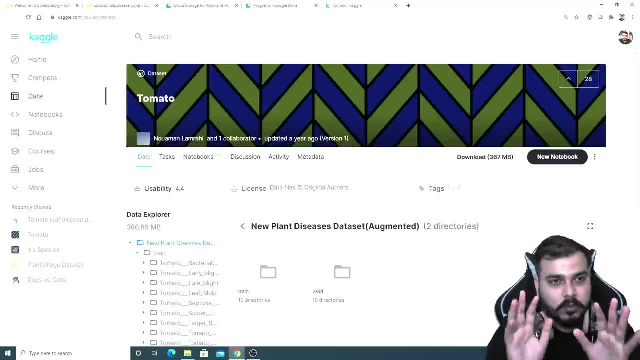 patient because it may take a little bit more time, But Google Colab is a boon for every students and for the people who cannot afford GPUs or heavy laptops or heavy workstations, So this is the way that you should try to learn. In my initial career of days in my data science industry, I have used Google Colab a lot, you know in terms of executing, training, your models and all. So in this particular video, I'm going to show you an example: how you can train deep learning models inside the Google Colab. It will be pretty much a 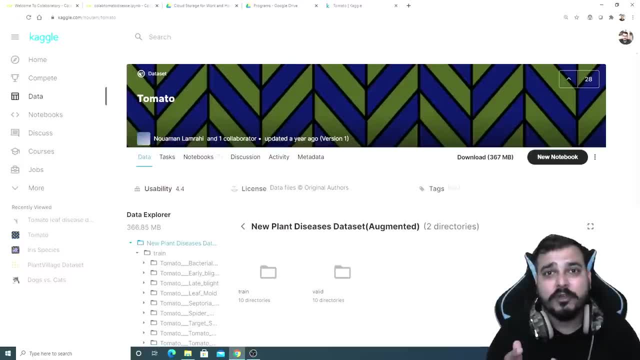 And just follow the steps that I'm actually going to say you And why this is important: because in the future, I'll be coming up with videos related to BERT and all, And probably that I'll not be doing in my workstation, because everybody do not have a GPU. So what I have thought is that, you know, I will be training them in the Google Colab and showing you all the examples, which is pretty much important, And this is one of the feedback that I got from some of my subscribers. So let's go ahead and try to, you know, train this particular deep learning model. 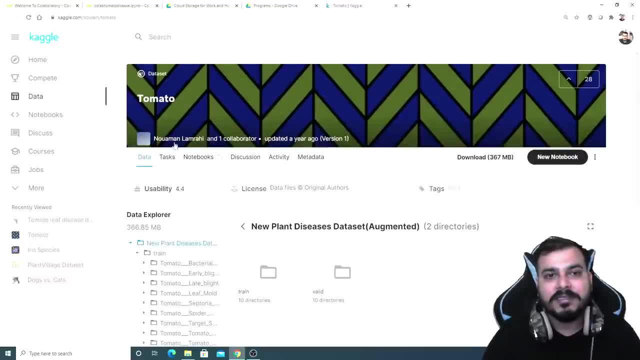 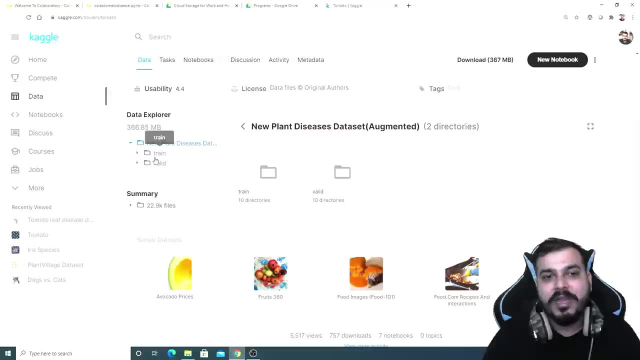 Now, in this example, what I'm going to do is that, guys, I've got a data set which is called a tomato leaf disease classification data set. Now, here you'll be able to see that in your data set you have the strain and valid data set. And you won't believe, guys, how many categories you have Here. you have somewhere around 1,, 2,, 3,, 4,, 5,, 6,, 7,, 8,, 9,, 10, 10 categories of different types of plant disease with respect to tomato leaves. So you can download this. this whole file size is somewhere around 367 MB. 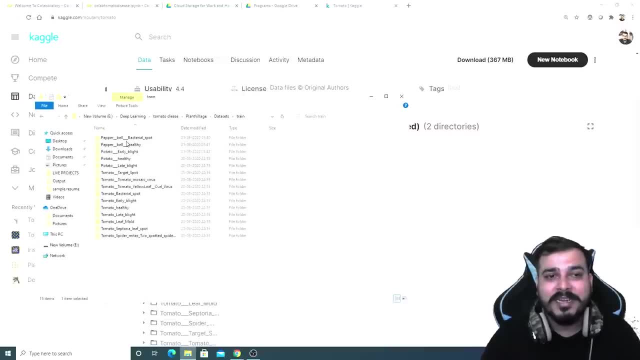 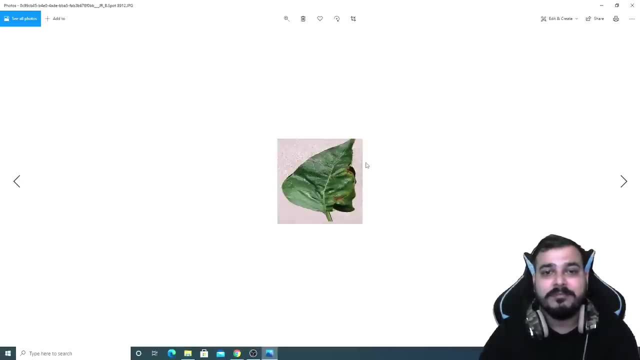 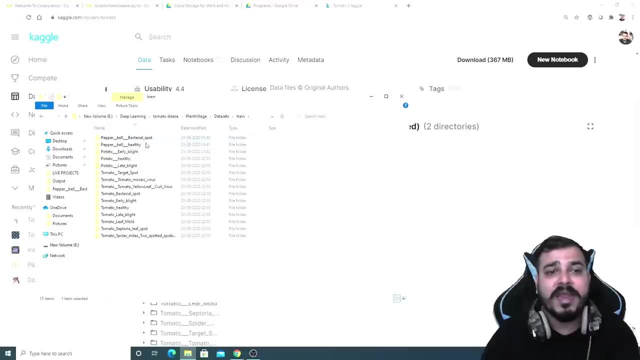 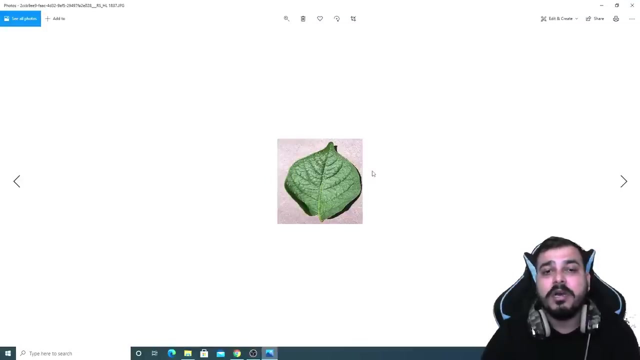 Now, and I have actually downloaded this particular data set. So here is all the images that you have. So if I open this images, guys, you'll be able to see all these images. So this is with respect to different different leaves diseases. So this kind of disease is called as pepper bell bacterial spot, Suppose, if you really want to see the healthy leaves. So this is what is the healthy leaves with respect to the tomato leaves classification. Okay, And apart from that, you also have different different things like 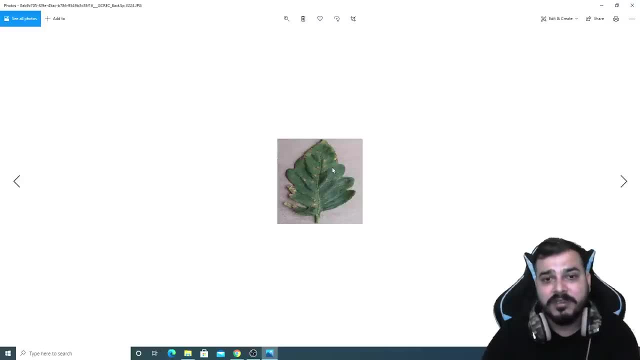 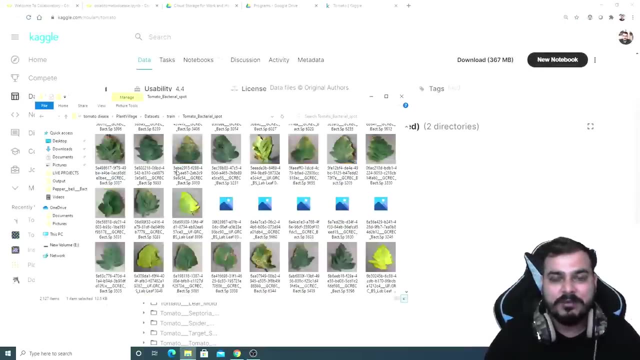 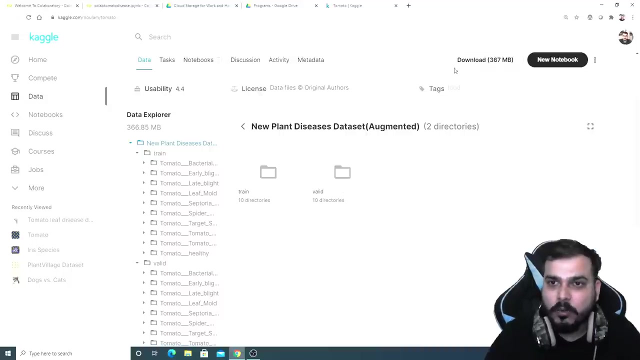 So here you can see this. all are the example of that. So it is nicely classified and really this images are somewhere around. I guess it is, it is, it is having basically many images. Okay, So let's see how quickly it will be done. So first thing is that just download this whole data set And Google collab. you know, first of all, this is the one way guys will be showing you, probably in the upcoming video that will be showing you more different ways, if na now you may. the way, guys, I'll be showing you probably in the upcoming video that will beiously showing you more different ways. If now you may be asking that, is it possible now that Google Collab has inserted a full, or do you have a single test at Google Collab and you're asking someone if someone with research voltar to Gord Nou is ready for Google Colab to apply for the test now? edit pro문 will cover you. 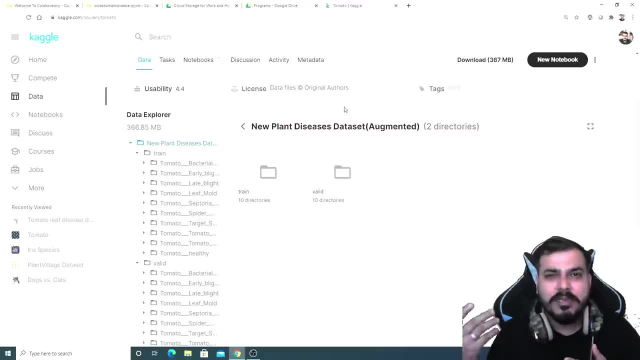 possible to directly pick up all the data sets from kaggle that all will be seeing in the upcoming videos, but this one is pretty much simple, so we'll download this whole data set. okay, once you download it, once it is saved in your local, okay, so if i take an example over here- so i had already shown- 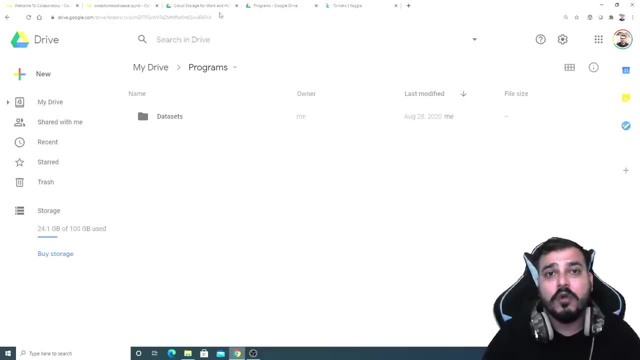 you that particular example. uh, then what you have to do is that just go inside your google drive and just upload this whole data set. okay, so you just have to upload this whole data set. you can see that i've uploaded all the data sets. i hope. i hope you have worked at google drive right. it is very 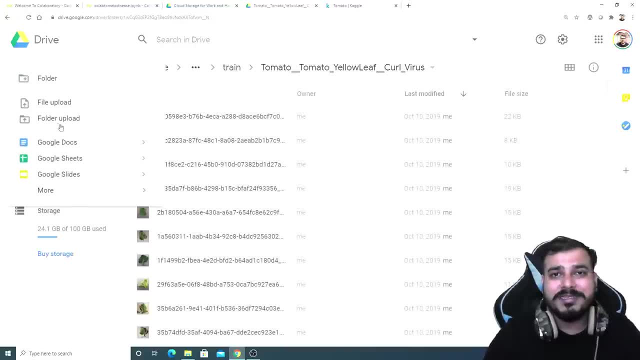 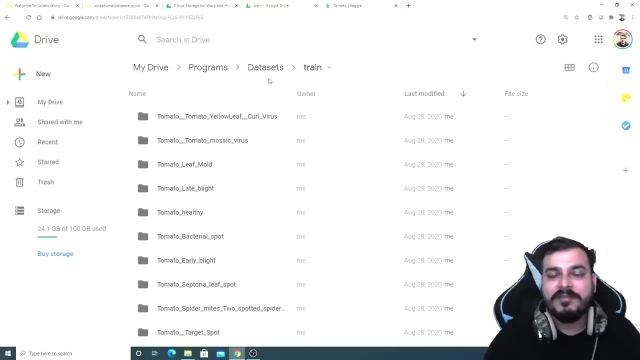 very much simple. you just have to click on new folder upload and just select that specific folder and, based on the path, you can actually save it. so i have my drive programs inside that, i have that data set and i have actually uploaded this train and test. okay, so this is what the data. 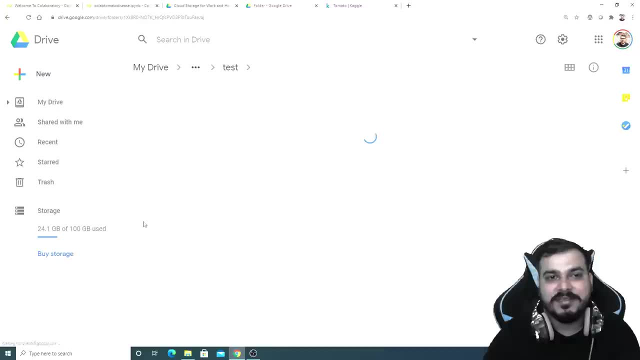 set is. so here you can see that all the data set is over here inside this, all the images also, you'll be able to see it. okay, so these are all the images. so this is the first step and since there are many images, so it may take some amount of time, you have to be patient, just. 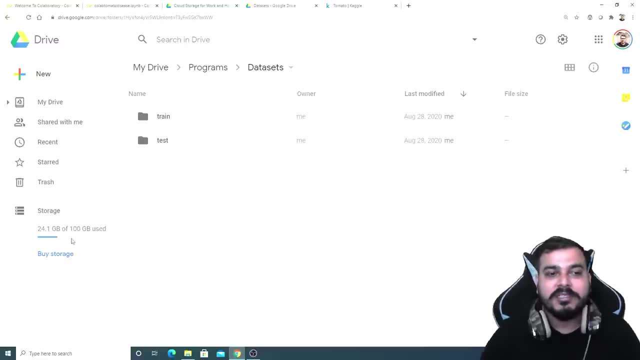 and it depends on your internet speed. i have also taken some additional storage of google. uh, probably the price was very much less, but i have somewhere around 100 gb which i'll be using for my personal purpose, like training models and deep learning in google collab and as you know. 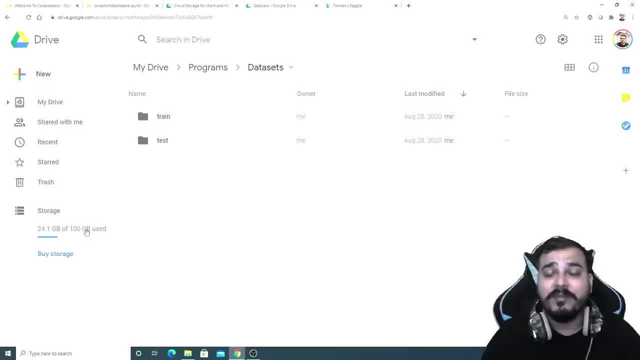 that i'm also coming up with playlist in bird, so that is the reason why i've taken 100 gb again. you can also take one tv, two tv, based on your requirement, and it is not necessary that you have to compulsory buy, but by default you'll be getting 15 gb. now you can see that i've. 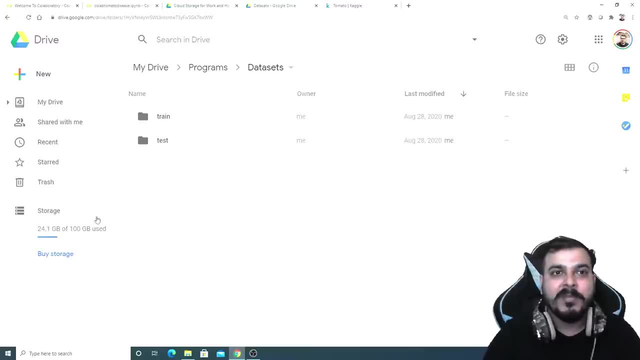 i've crossed the 15 gb mark. i have somewhere around 24.1 gb. okay, now the first step you have already done: just upload this whole data set. then the next thing is that just open your google collab. okay, so, google collab. now what i'm going to do, the reason why i put all this particular data set. 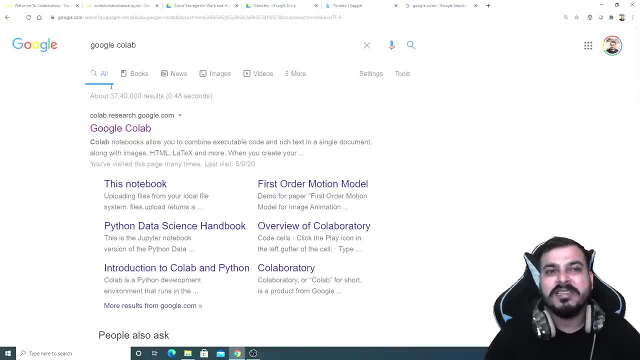 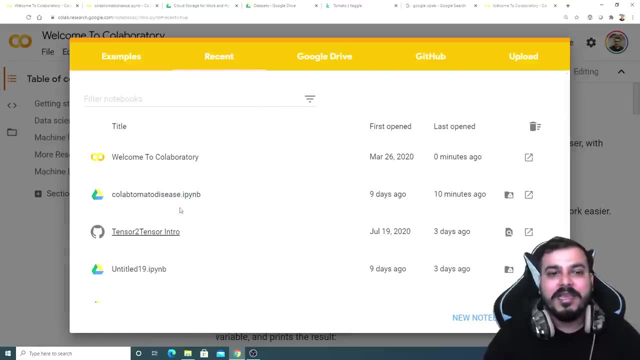 inside the google drive, because i'm going to use this data set and call it inside my google collab. so just go and open the google collab. so here you can see that i have created one ipainb file. if you have not created the, just create, go on. 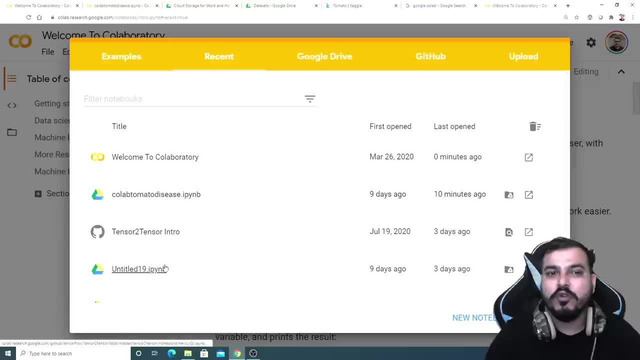 creating new notebook and just click on this and a new notebook file will get created. so right now i'm just going to open this collab tomato disease ipminb. this is also getting stored in the google drive itself. you can also take it from github. you can also upload. you can also upload this, ipynb. 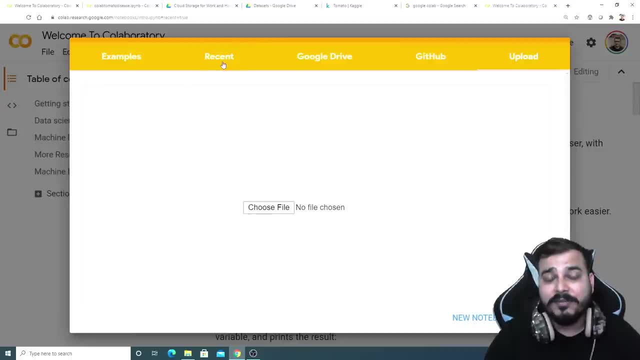 file by this particular option. okay, so suppose, if, uh, and definitely, i will be giving you this particular file in the github. so what i'm going to do is i'm going to go to my google drive and i'm going to go to my github. so what you can do, you can either load it from github or you can also load. 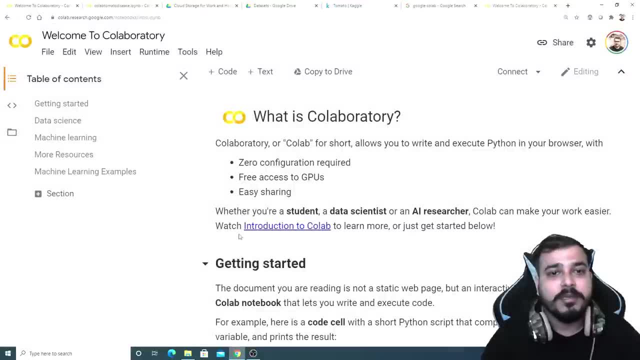 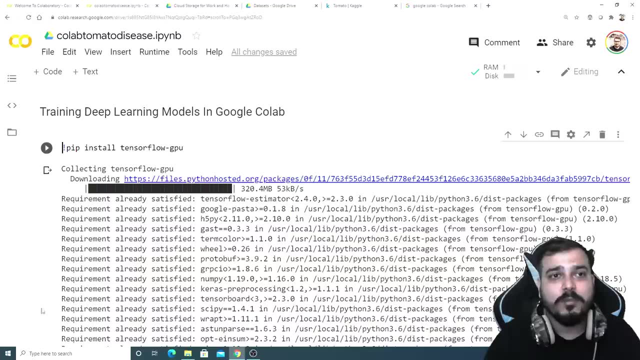 it from upload section, right? so this is pretty much simple. now the next thing that we are going to do is that: um, okay, this i'm just going to close. just imagine that i've opened this particular file. now this is the whole code that we are going to run, and sometimes i'll just tell you what. 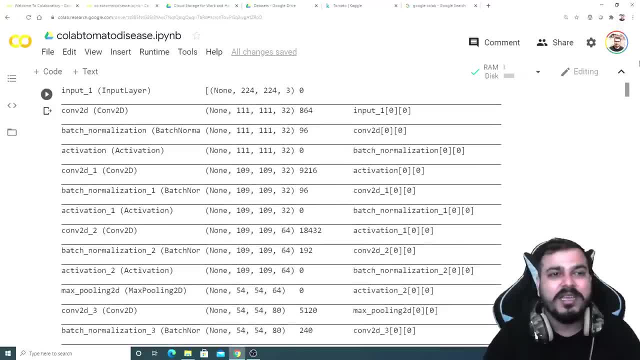 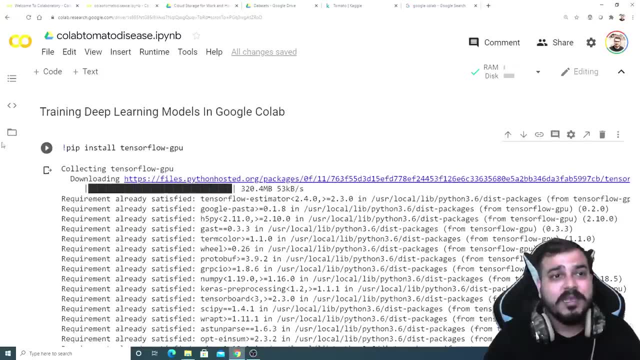 are the steps and this particular code. i have also explained in different uh image classification problem statements and how do you train your model and all. so don't worry about it, i'll be showing you all the steps now, as soon as you open this. just click on this particular folder. okay, 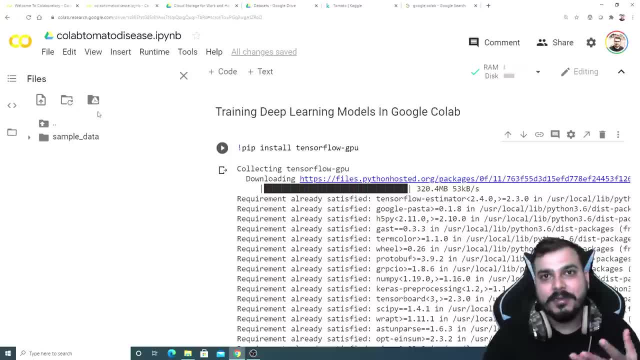 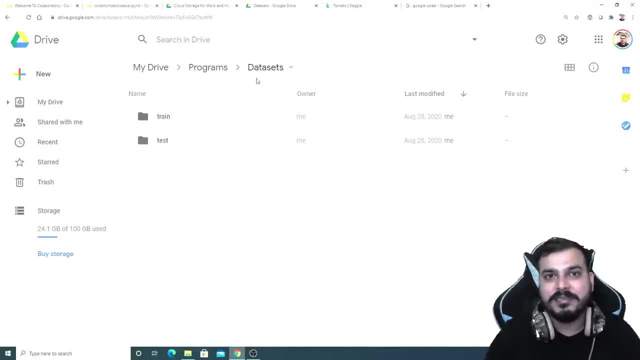 now, when we click on this particular folder, i have to connect to my google drive. the reason why i have to connect to my google drive is that because i want to access this particular data sets. right, i have to access this particular data set, so that is the reason i have to import this particular. 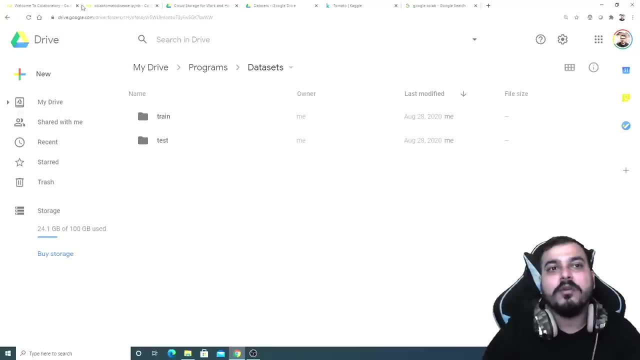 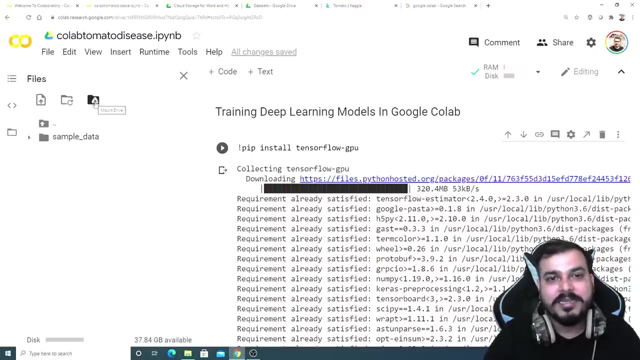 data set, or i should be able to read this particular data set in my google collab itself. so for that, you will be seeing one icon over here which is like this: okay, so just click over here and it is nothing but mount drive. okay, this is pretty much important before. uh that, guys, i let me and 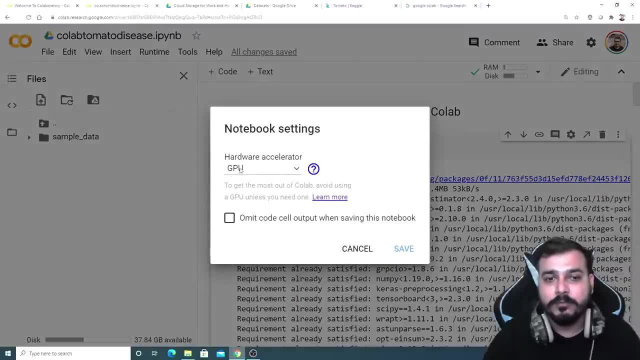 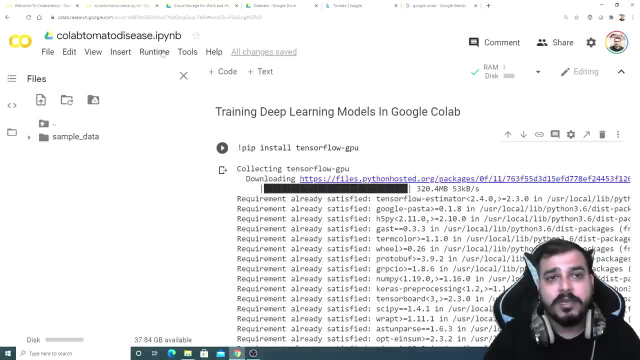 you have to also do this. you have to change your runtime to gpu. okay, uh, initially it will be none, okay, so make sure that you change the runtime to gpu. so if i go and see my runtime it is already gpu, so i'm not going to change it. but you just check what your notebook setting it is, whether 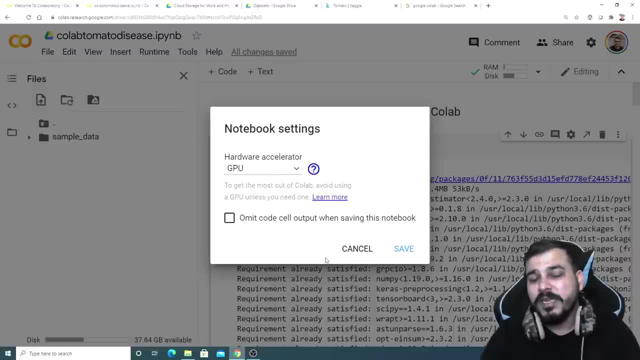 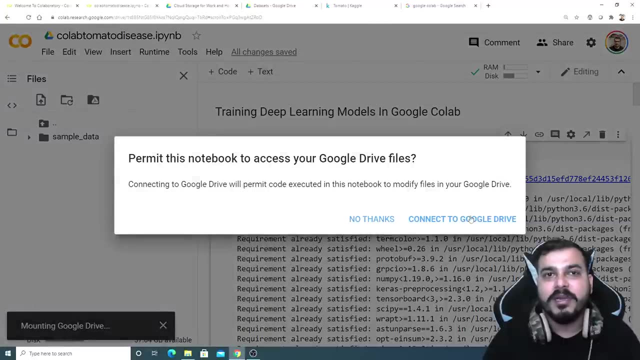 it is in gpu, tpu or none, but make sure that you make it in gpu, okay, once you do that now the next is that you have to click on mount drive. now this mount drive will be asking the permission to connect to your google drive, so that basically means you need to be in sync with your google. 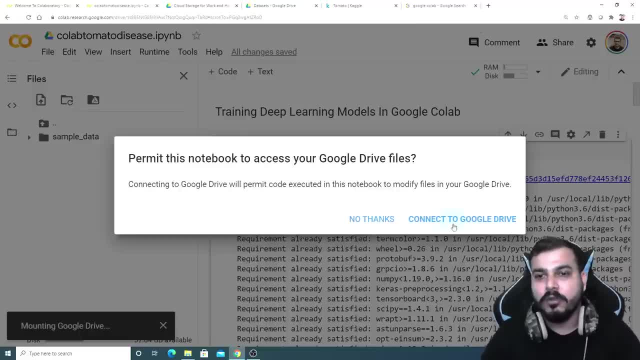 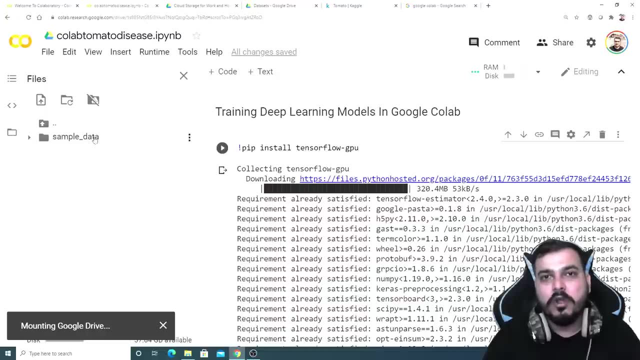 basically you need to log in in the google inside the browser. so i'm using google chrome over here, so once i connect to google drive- it will take some time- you'll be able to see that now there will be a folder which is called as drive, and this also file folder is there, and these are: 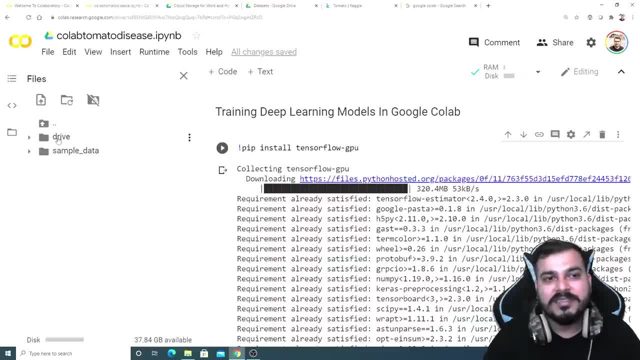 the basic data set that is already present for practice purpose. now you can see that there is a drive folder that is coming, and now, if i open the drive folder inside my drive, you'll be able to see the path. uh, these are some of my personal documents, so. 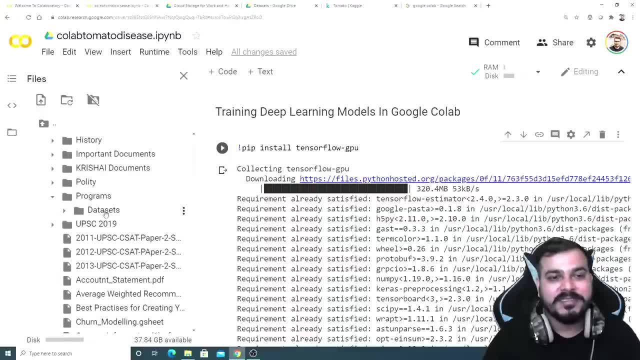 ignore that. so inside programs you'll be able to see data sets. okay, so here you'll be able to see data sets. now what you can do is that, if you really want to find out the path of the data sets inside this data set, you have test and train. so if you really want to know the path, just go. 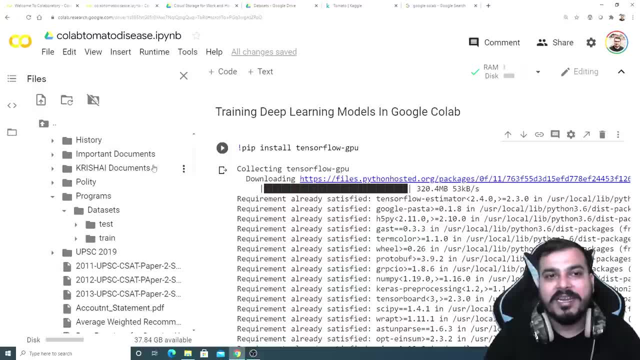 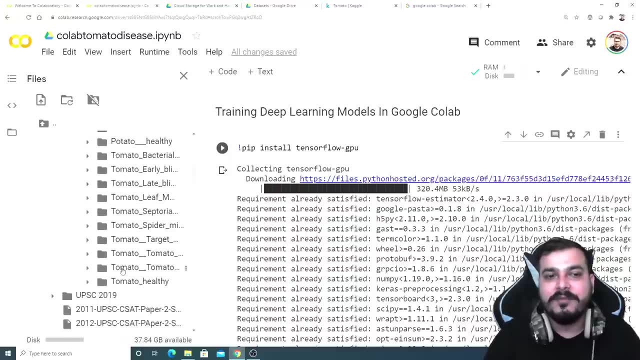 right click and just copy path. okay, so when you do right click and just copy path, you'll be getting the path of the data set. then you can write slash train and slash test and then when you click on test then it will create the images. so these are having all the 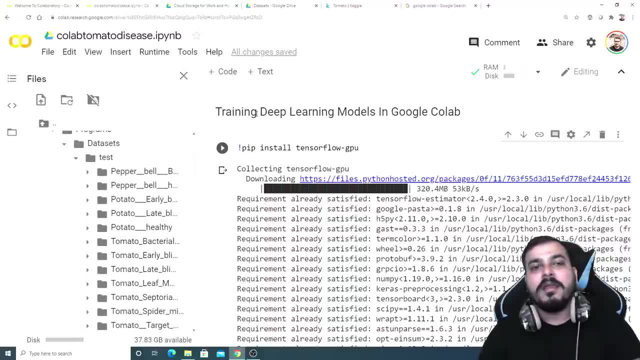 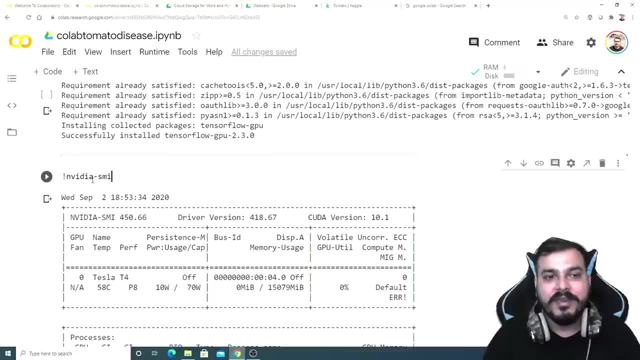 images over here: train data set and these are having the test data set. so i'm just going to keep it over here. now let me just close this, and the first step that you really have to do is that i will go and execute this slash nvidia, that slash smi, so this will actually help you. 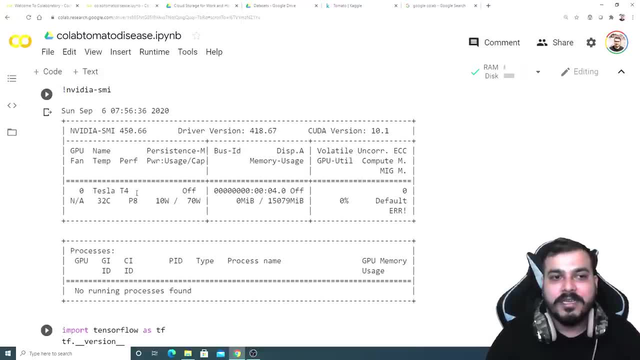 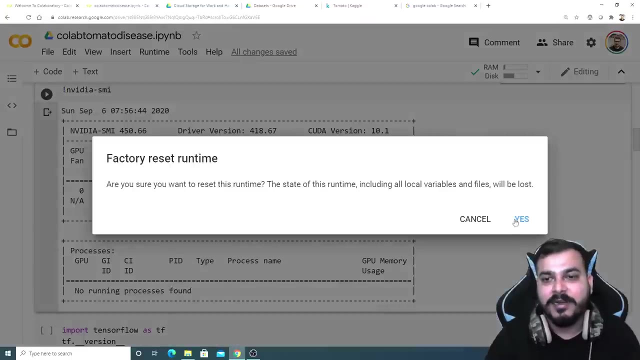 to understand like which gpu has been allocated. so here, uh, it is written tesla t4, so just try to execute once again. okay, and there are options. sometime you'll may get tesla t4, sometime you'll be. so if you really want to change the GPU, sometimes you can also do a factory reset. factory set run. 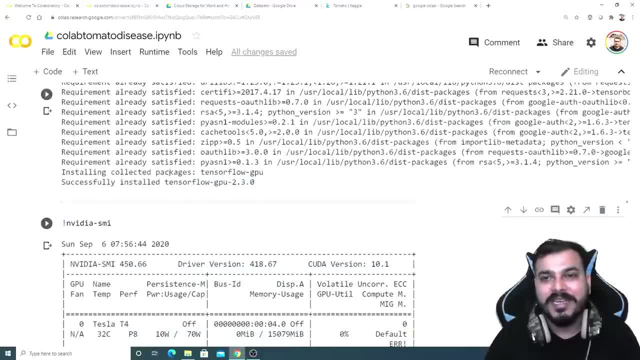 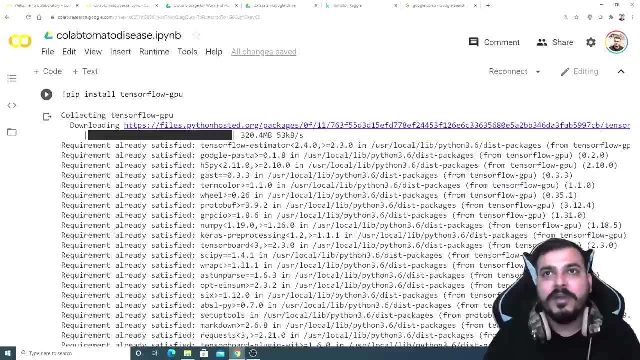 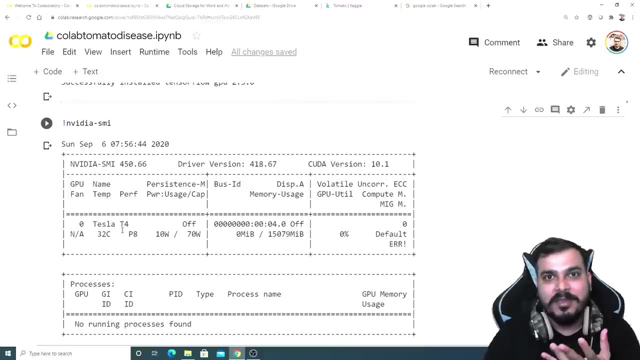 time and after that, probably you will be again getting, or you may get, another GPU, but most of the time you will be getting Tesla t4- even in one of my video where I had actually explained you about rapids AI. so there also, the requirement is that you need to get Tesla t4, okay, or some. 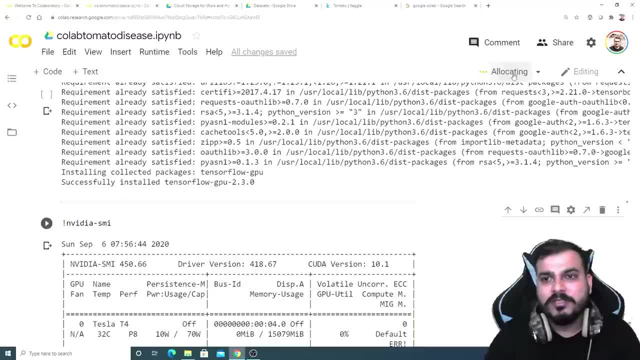 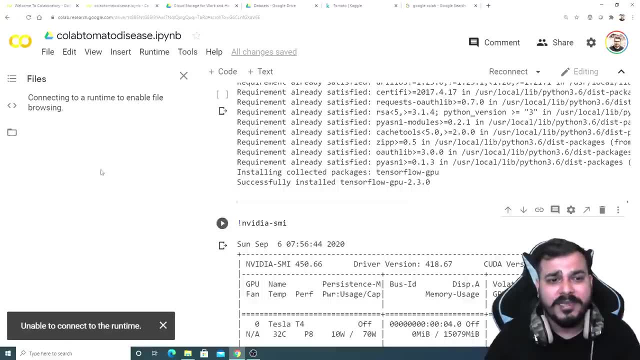 other higher GPU. other than that, it will not work. so I'm just going to connect on really connecting. so let me see whether my drive is there or not. again, it will be coming over here. it is initializing. it is saying unable to connect, but don't worry, it will be mounting the Google Drive. 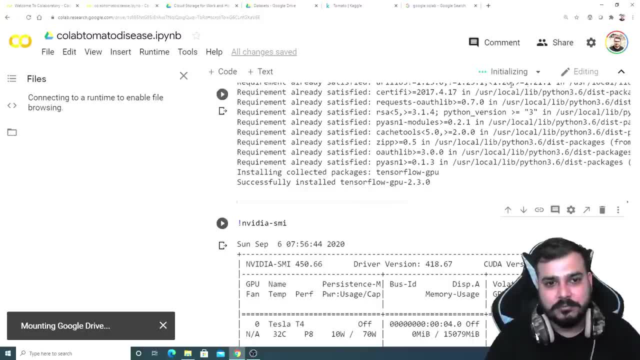 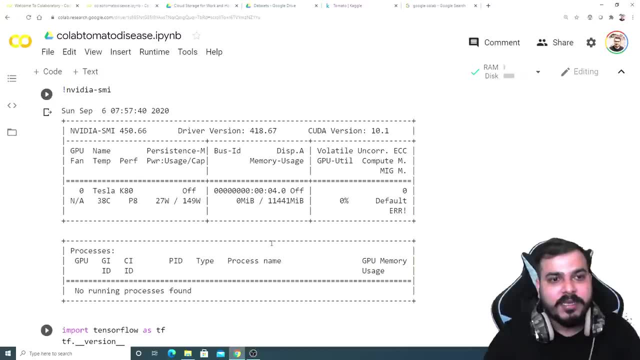 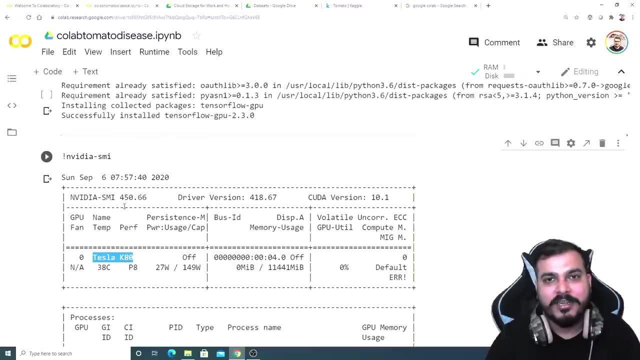 automatically as soon as it is connected, and it may take. it may take some time, definitely. so, yes, it is connected. my Google Drive is here. I'm just going to execute this again and let's see whether my GPU will change or not. so now I have got Tesla kat. okay, so it depends, just try. 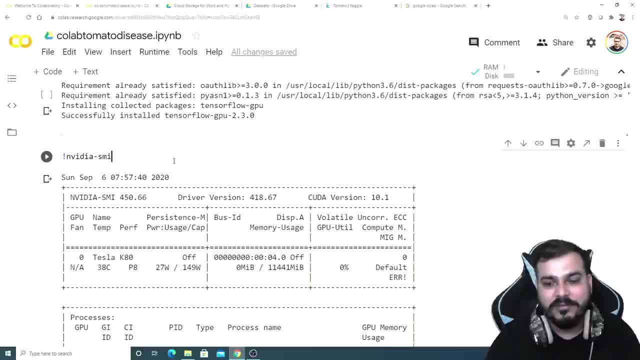 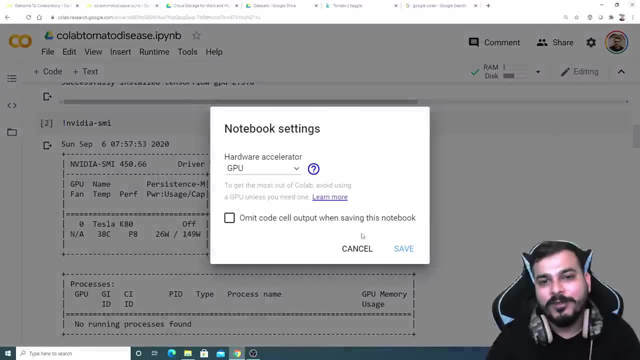 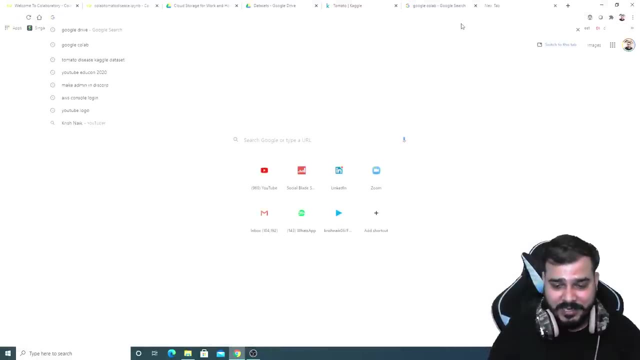 to find out that gpu is better for you, whether tesla t4 or tesla kat, i will just execute it again. so right now i'm getting tesla kat. suppose i really again want to change the run time- sorry, not run time. suppose i could do factory reset time. and if you don't know about tesla, tesla kat, so if you can write. 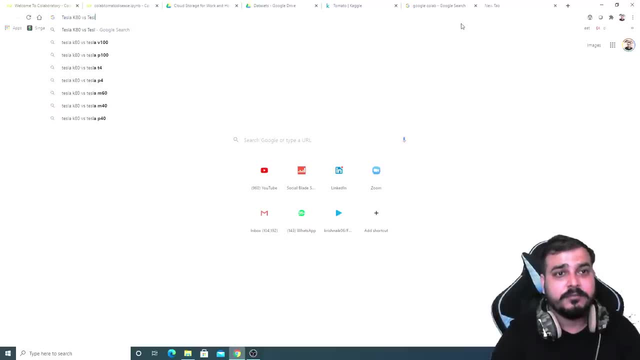 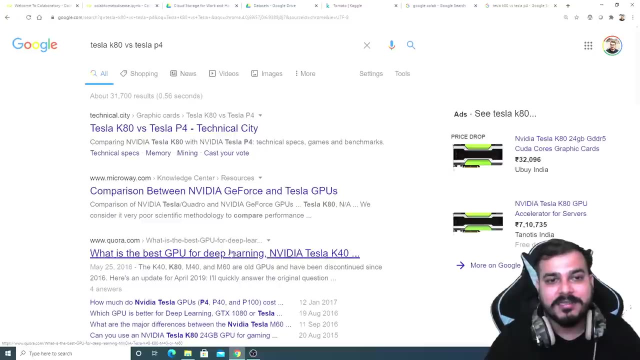 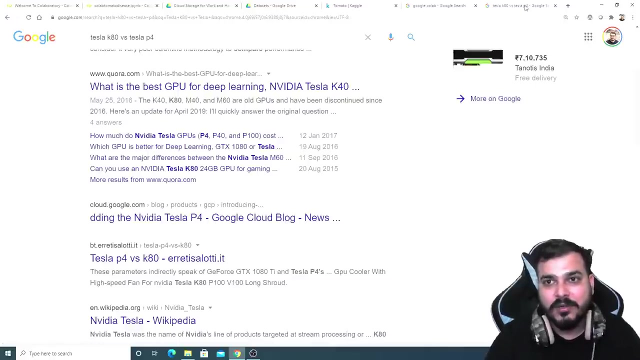 tesla kat versus tesla- uh, i think it was t4, right or p4- which one is better? you can see this inside this url and, uh, select those which is better. okay, suppose, if tesla kat. i think tesla kat is not that good when compared to tesla p4. so again, i have done this particular step. okay, so again i'm going. 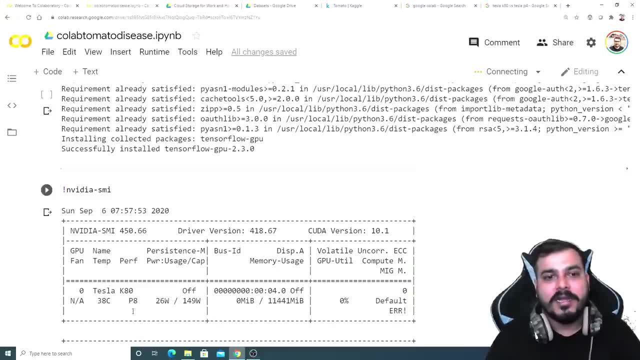 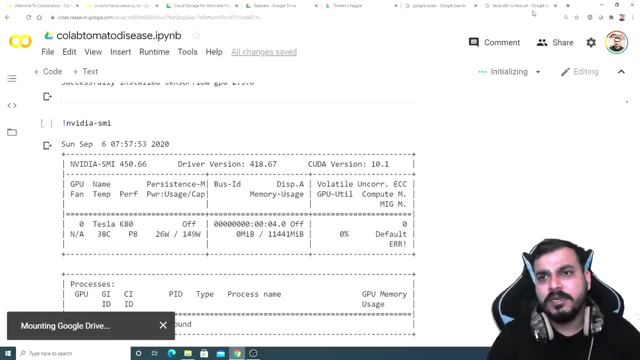 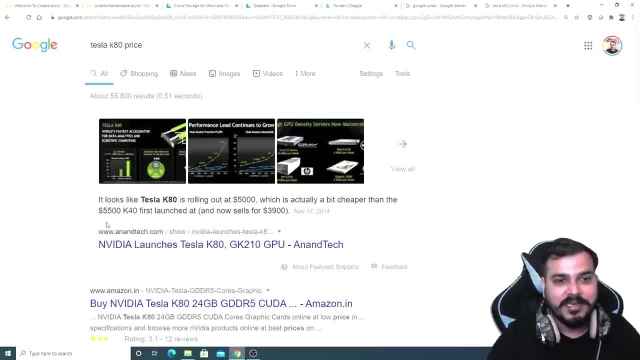 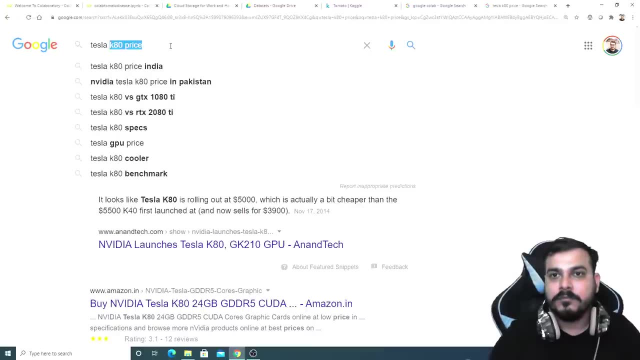 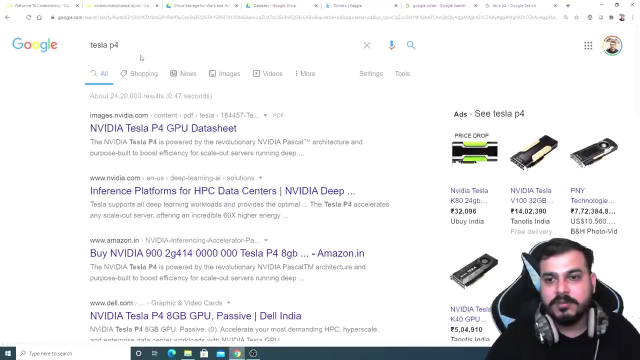 is performing better. just find out the price. tesla kat: uh, tesla kat is rolling out at five thousand dollars, and probably tesla p4- right p4 cost. so okay, tesla k 80 24 gb is somewhere around 32 000 inr. 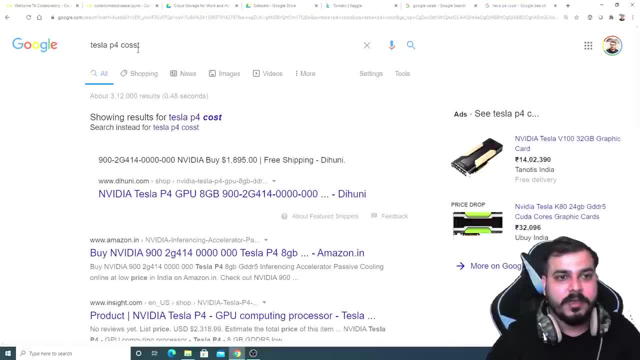 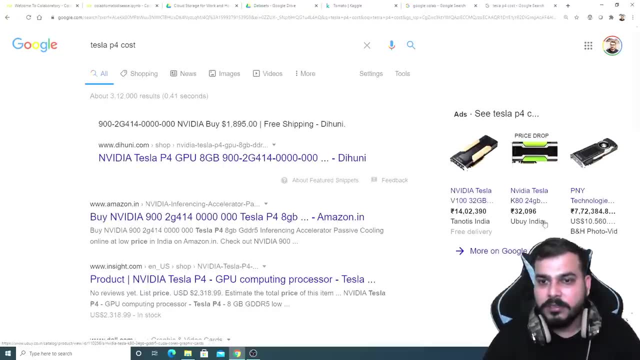 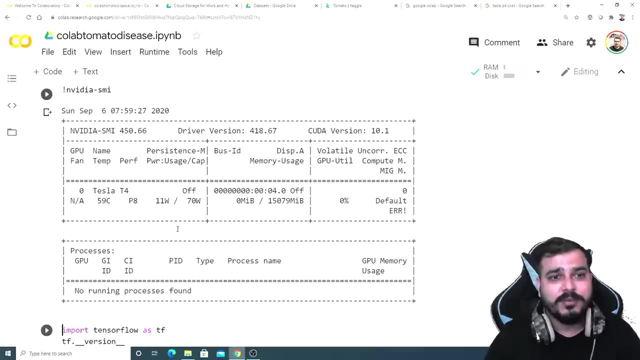 okay, and this cost is somewhere around. let's see how much it is, i don't know, let's see. or tesla t, tt, t, t, but i think tesla k80 will not perform that better. so this is connected. let me just execute once again and see which gpu. now i've got tesla t4. sorry, i was selecting at t4. 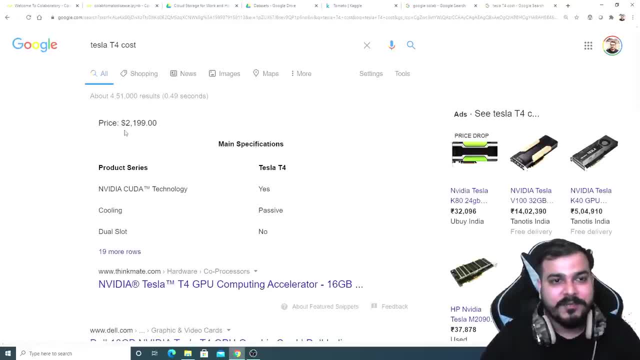 so let me select t4, okay, so this is somewhere around two thousand one nine nine dollars, which is better than at least tesla kat. that is 24 gb, that is 32 000, but i think, uh, we should, we will go ahead with this, okay, so once i execute this, uh, 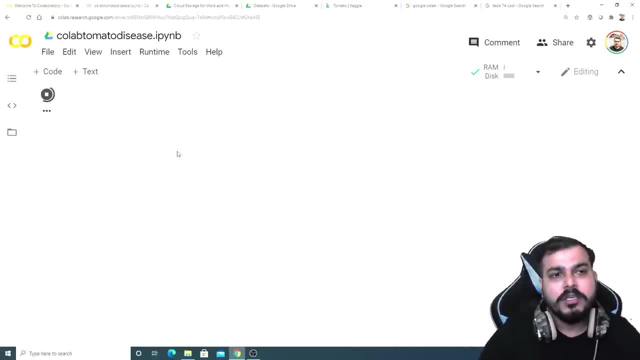 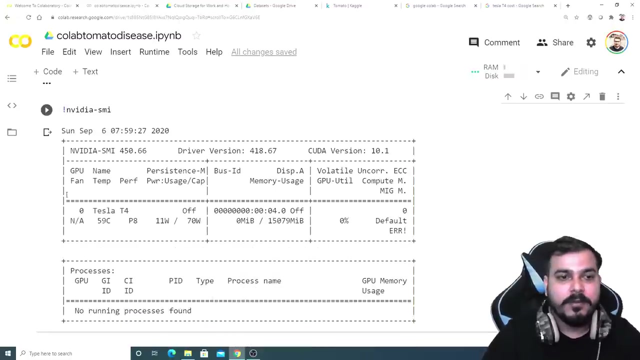 the first thing that you have to do is that install the tensorflow gpu. so for that you can write: uh, exclamation: pip, install tensorflow dash gpu. sorry, it was tesla t4 i. i used tesla p4, right, i don't know. okay, so tesla kat versus tesla t4. uh, you may also get some other gpu. 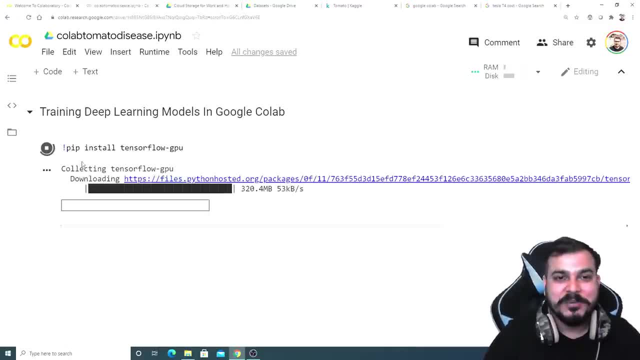 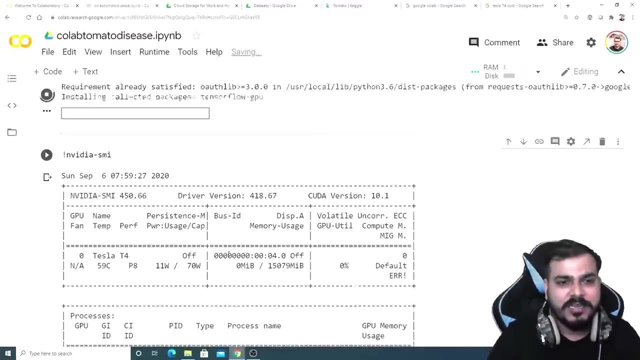 allocated. uh, it is upon your luck and basically upon the usage that people are using, but every time if you do a factory reset runtime, some other gpu will get allocated to you. okay, so probably it says a requirement already satisfied, because i had done already everything so installing, collected package, tensorflow, gpus, and remember, guys, the tensorflow version that we 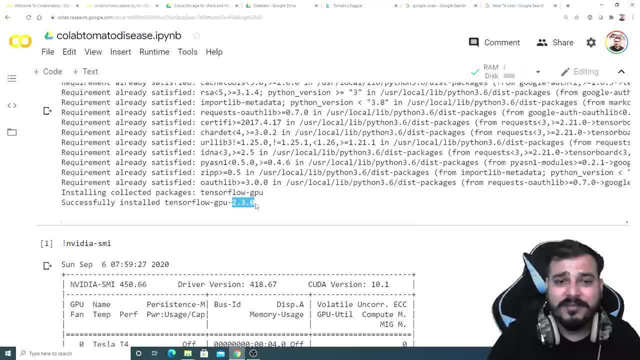 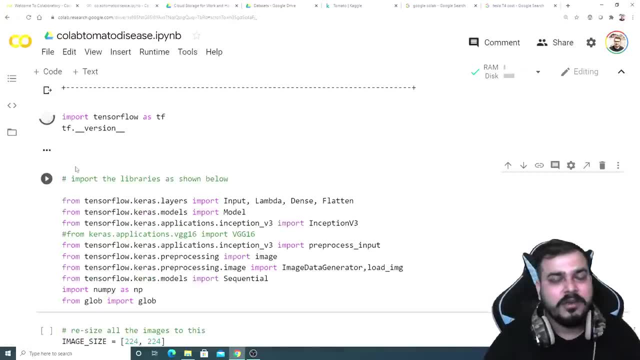 will be using will be greater than so. here you can see that it is having 2.3.0, the most recent one, so this has got executed. perfectly fine, guys. so if you really want to see the version of the tensorflow, so here it is 2.3.0. now one more thing that, uh, i really wanted to show. this is basically your ram. 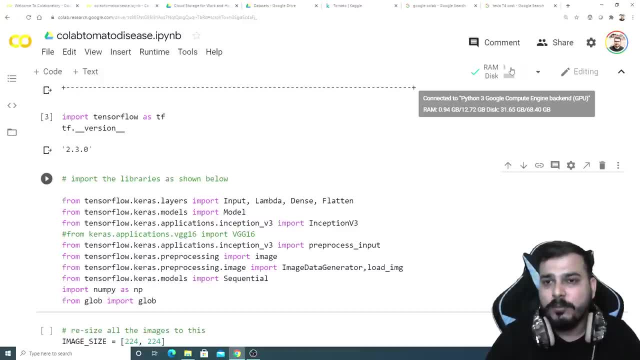 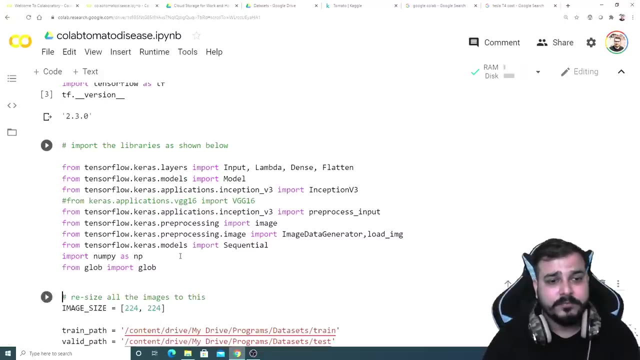 okay, so the ram overall size, i think it is 12.72 gb. uh, the hard disk size is somewhere around max is somewhere around 68.40 gb and i think 31.65 is getting used right now. let's see. okay, so after this i'm going to execute this. uh, this is all my installation. i mean all the libraries that. 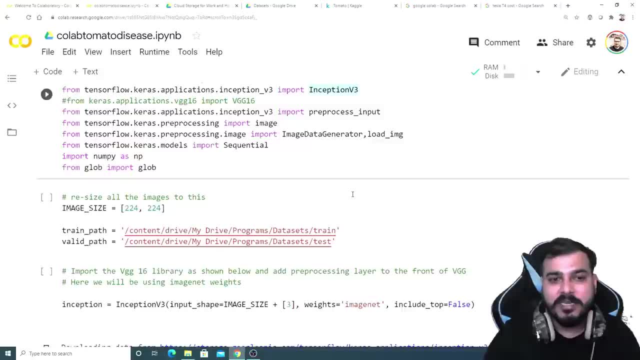 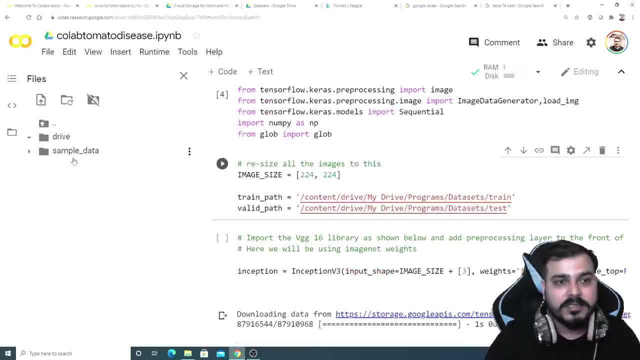 i want to import, and in this case i'm going to use inception v3. uh, after this, uh, this is pretty much important guys: the training and the valid path. right, as i told you, the training and the valid part. so suppose i will say that this is my programs. okay, my data set. my train. okay, my train. 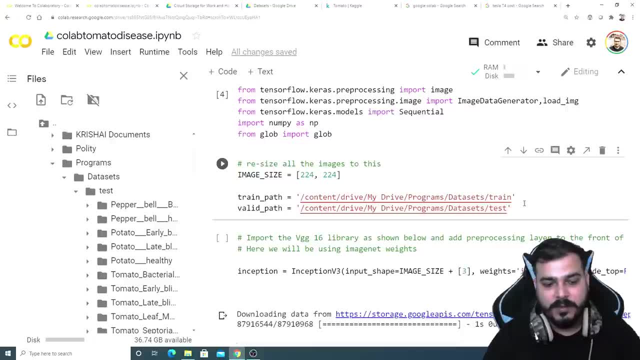 if i want to give this path, i'll just copy this path over here and here. if i paste it, you'll be able to see that this whole path is available for the test, right? so i will just be using codes and this path will get selected. this is how you have to select your. 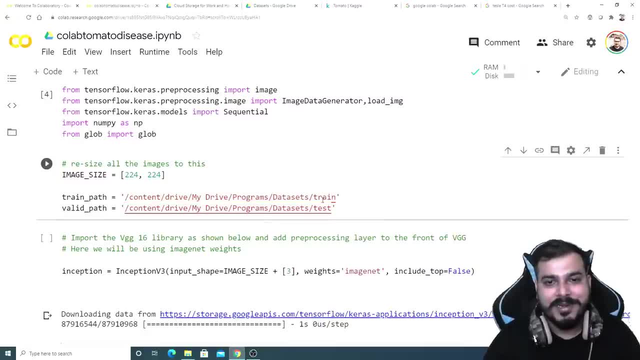 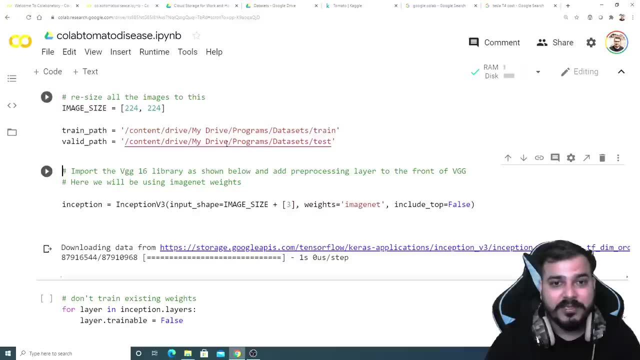 path. okay, so this is done. and similarly, you find out the train path and test path just by clicking click and you'll get the path. after this, this is the path of your data set, so please make sure that you have this is correctly. otherwise, if you are running in your local, you just have to give the 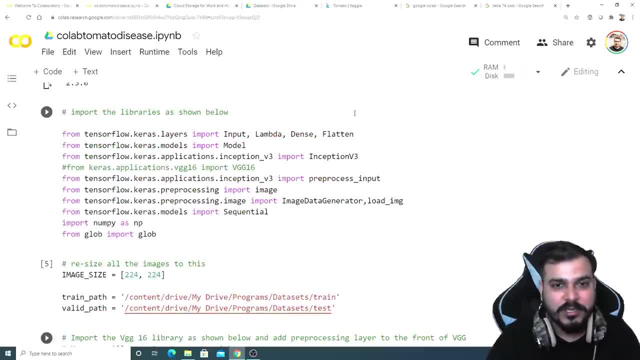 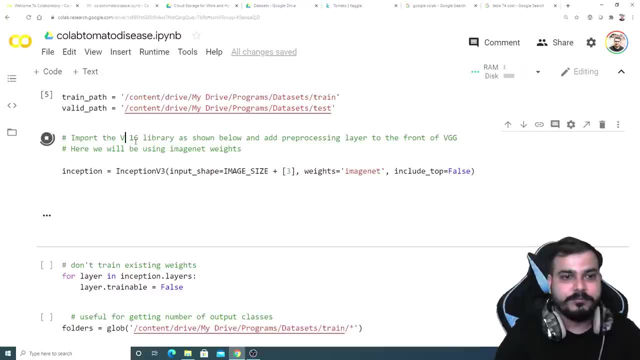 path and this is a transfer learning technique. guys, here i'm actually going to use inception v3, so let me just import inception v3 over here. sorry, this should be inception v3, inception v3, not. oh. so here you can see that downloading data from this, this, this, this and this has got perfectly. 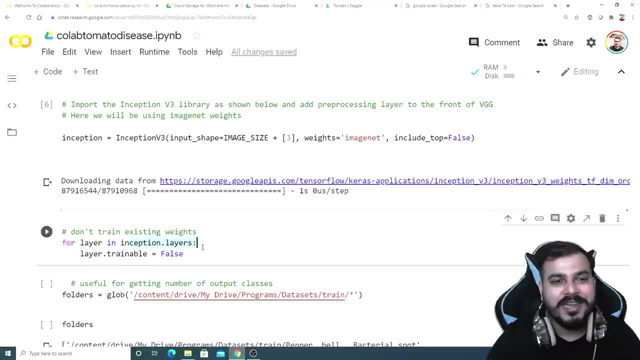 executed, then the next step what i'm doing is that i'm making all the layers as false. okay, and this i've explained in my previous deep learning videos also. so for layer in inception dot layers, layer dot re-enable is equal to false, because i'm using a transfer learning technique. 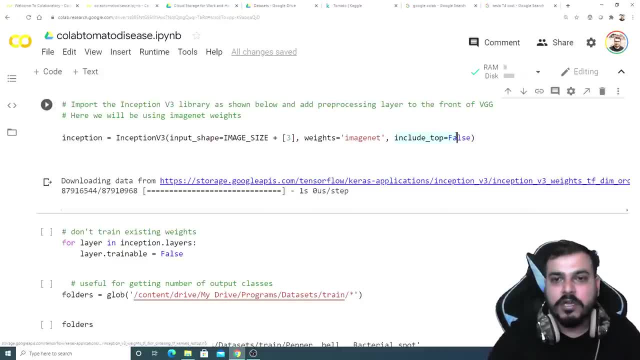 i want to use all the weights. and remember, guys, this include underscore top is equal to false. this basically says that i don't want to use the first and the last layer, so because of that, i'm actually using this. so once i execute this, this is done, i really want to get how many output classes i need to. 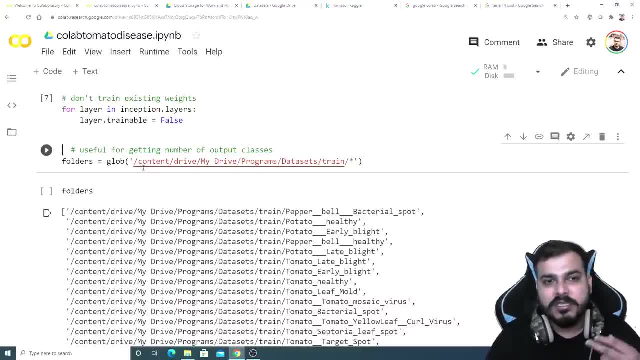 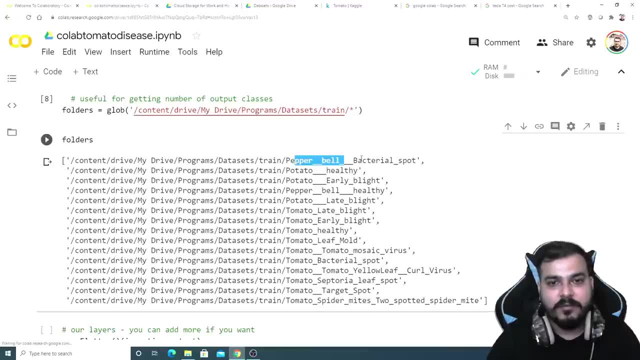 have, and that is basically. i'll go and check inside my train folder to see that how many classes are there. so this is basically my folder size, so i'll be getting all the folders. so definitely, in this case, this is my folder and length of all this folder will basically be the. 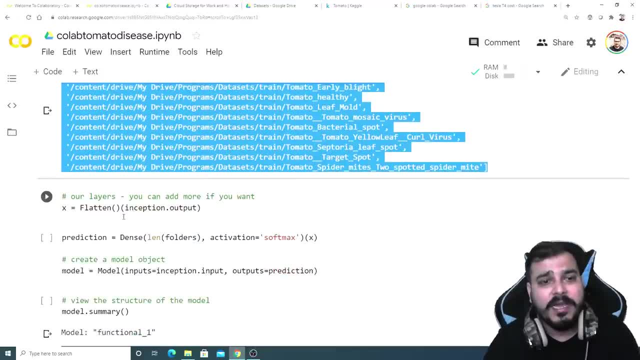 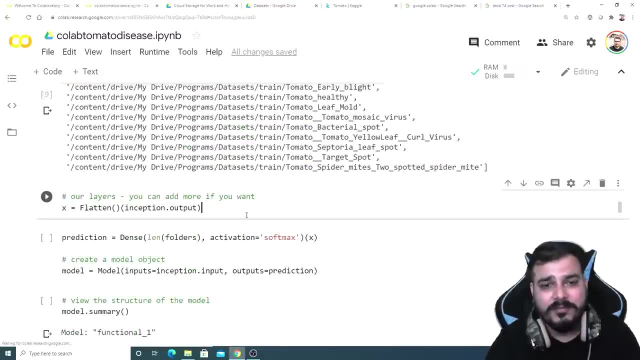 number of classes. okay, then over here i i'm flattening all the output of the inception that i've downloaded over here, because i'll not be having the last layer. you after that i will be adding my custom, custom number of this length of folders. basically says that: how many is the output node that you want? right, and for that i'm using this dense. 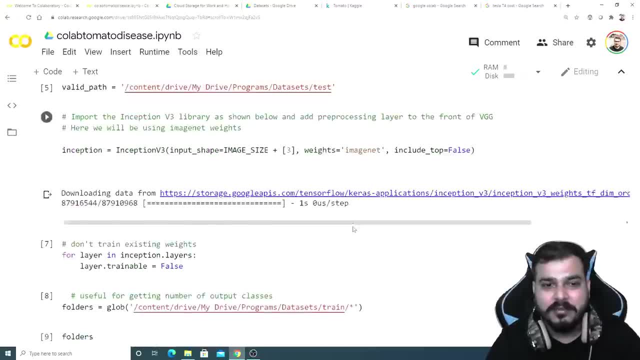 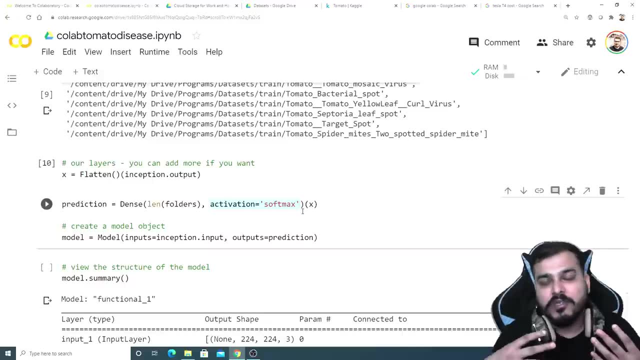 dense. i've imported it over here: right, dense and flatten. so that is done. so and yes, i have to use the activation as softmax. remember, if you just have a binary categories, you can use uh. if you have two categories in the output, you can use sigmoid. if you have multiple categories, you. 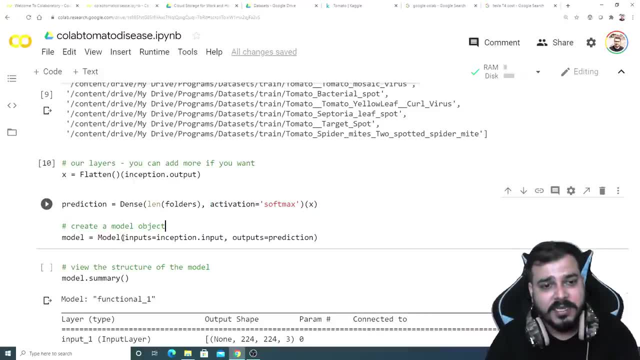 should go with softmax. okay, so this is done and here you can see that i've added my custom number, that i have put to the last rate of tierra, just to do this. you can see, with slut inspiration from last class. you can see that i'm creating a model object with inputs as inception dot. 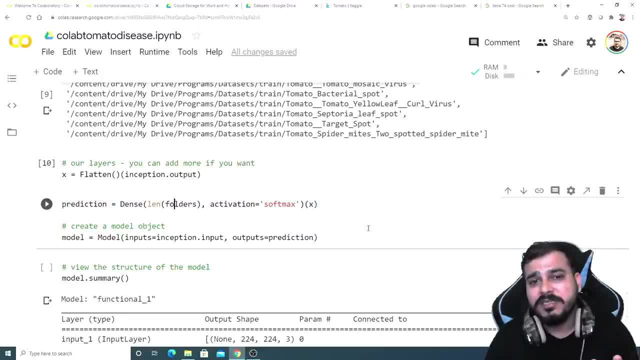 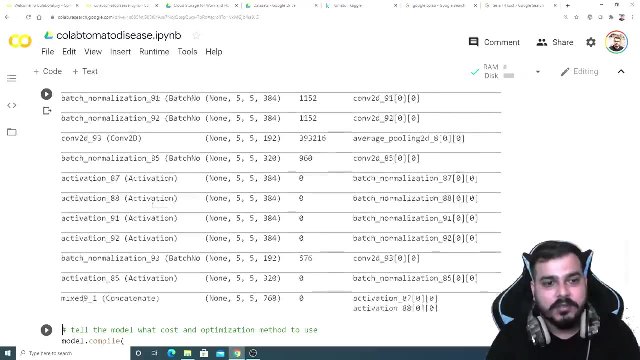 input and the output as this particular prediction that i have, and in this prediction i have 10 nodes as my output and the activation function is softmax, along with concatenating with the flattened layer of the previous inception. so once i execute this, this is god and modelsummary. so this is how it is. uh, you have to focus on the last layer, guys. last layer is: 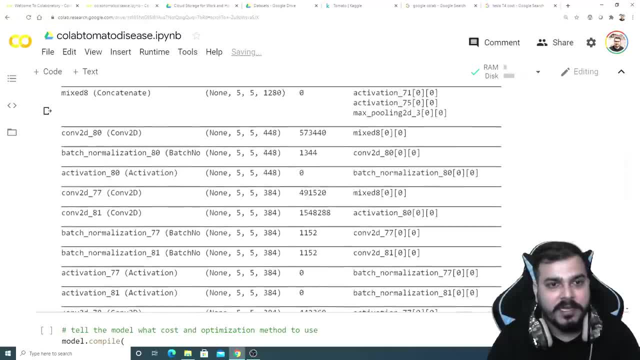 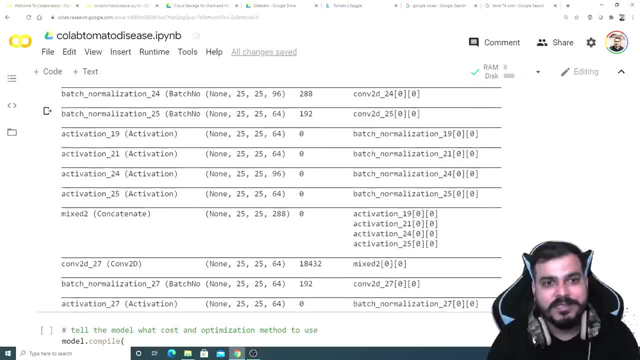 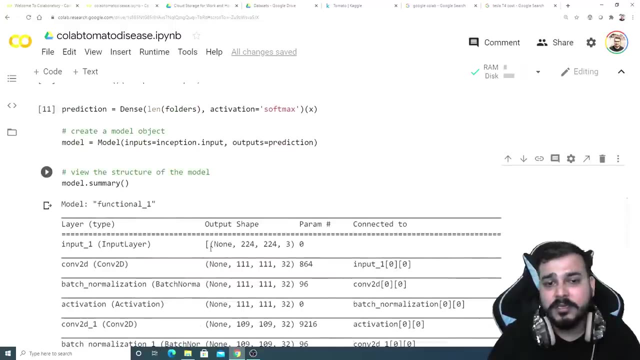 15 layers, okay. so probably i think inside the train we have 15 layers. okay, and in the first layer also, you have to actually see, okay, inception v3- just go and check the architecture guys, how it is, but it is a very, very big layer. so in in inception, in the input layer, you can see 224. 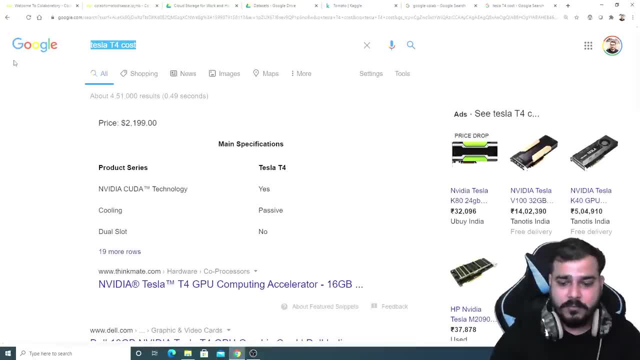 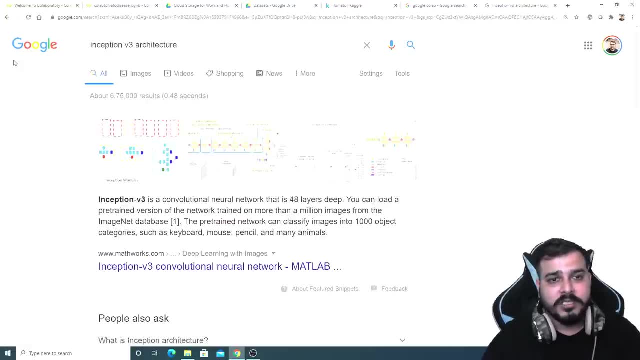 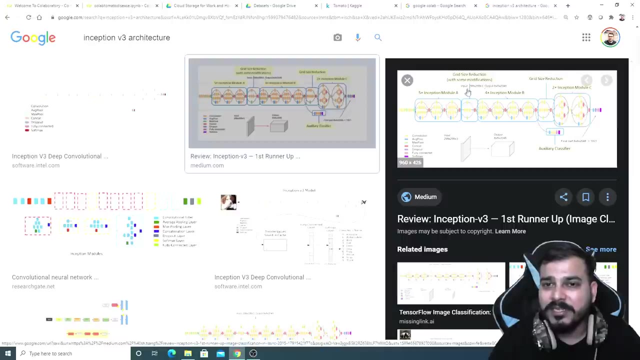 comma 224, comma 3. so if i go and search for inception v3 architecture, so if just let me know if you really want to understand all this particular architecture, guys, i can also create a video. so this is how an inception v3 architecture looks like: module a, module b and module c with 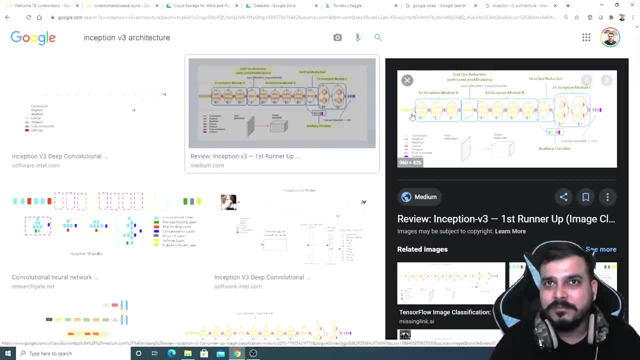 grid size reduction and, apart from that, you'll also be seeing- uh, no, that is interested in, sorry. so this is how the architecture looks like and you what all things are used: the convolution, average, pool, max, pooling, concat, dropout, fully connected and softmax. so these all are things are actually used inside that. uh, let's, let me create a video. 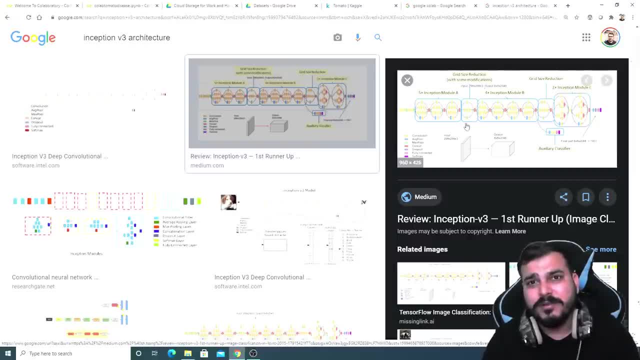 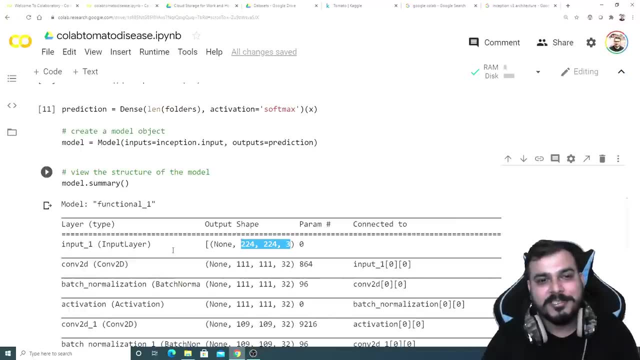 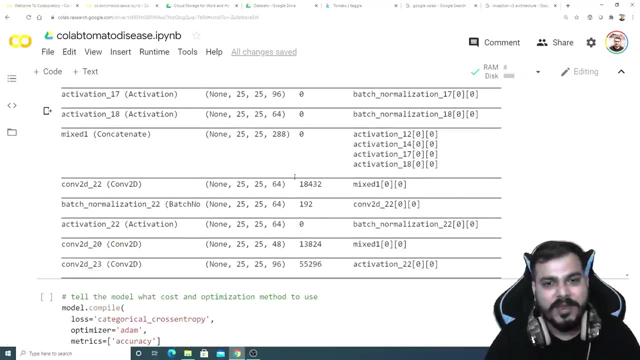 on all the transfer learning techniques. that will be also very, very helpful to you, because you'll be understanding the architecture. okay, okay, perfect, because anyhow, apart from that, you just have to use the trained weights from keras. right, i think that will be pretty much easy, okay, so we? 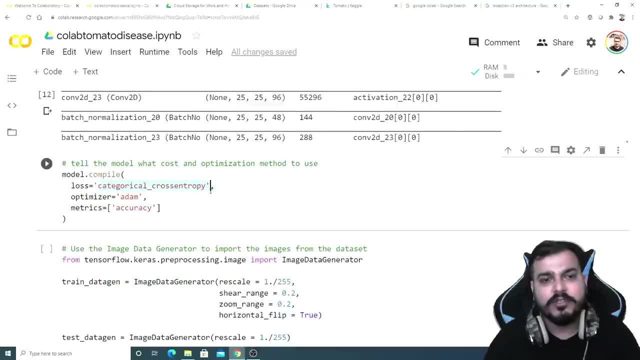 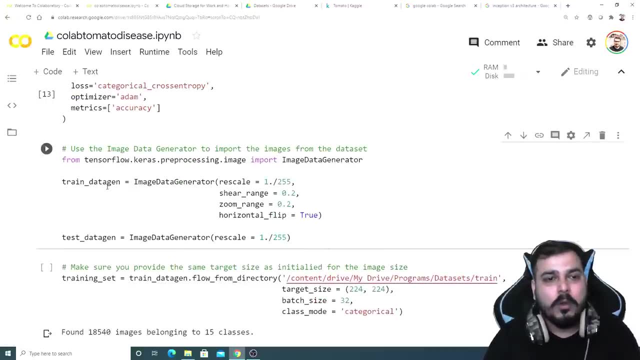 have done this. uh, next step is basically compile, and here we are going to use category cross entropy along with adam, and the matrix is accuracy. i think this is pretty much common for everyone. now, this is very, very important, guys, for the training data set. i'm applying these scaling. 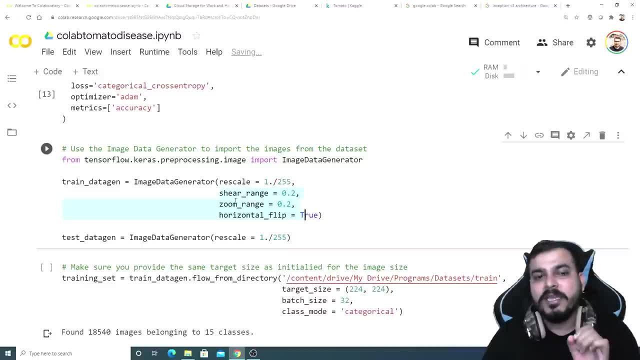 options, share range, zoom range. these are for the data augmentation and make sure that you have to scale down. it is pretty much important for the test data set. we don't have to do all these things because there we will just be doing scaling options. okay, so scaling option is done over here you can. 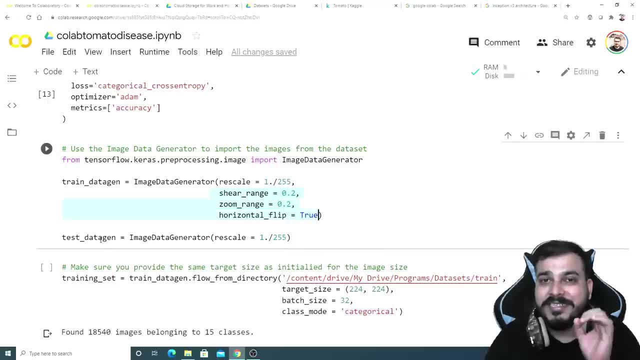 see ongoing scaling options. get down plano or CTLA scaling options. get down: now the scaling option is done, so scaling options get done. here you can see, don't apply data augmentation techniques in test data set. only apply the scaling one, okay, but in training data set you have to apply all these things. so for that, this whole, 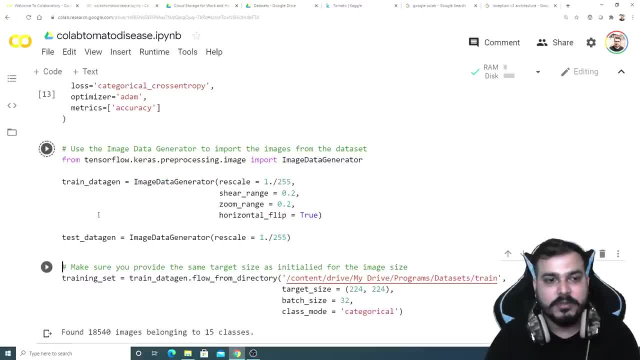 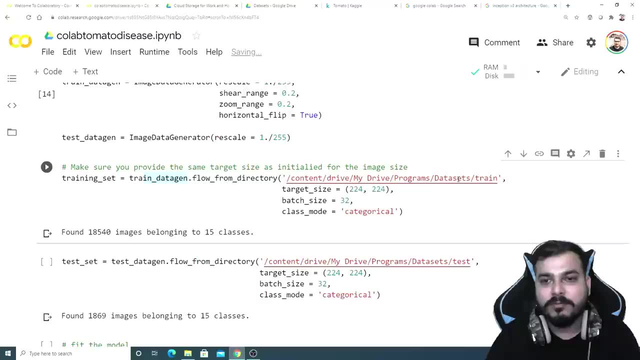 library is basically image data generator, so i'll be executing this and now i will be reading all my train data from flow from directory from this particular path, that is content drive. my drive programs. data set is slash train. the target size is 224- 224. batch size is 32. class mode is categorical. make sure that you provide the batch size as 16, because 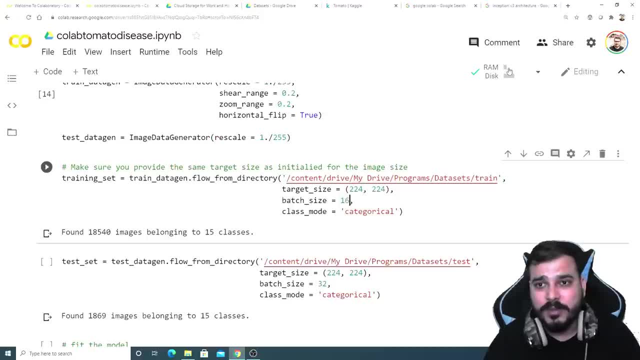 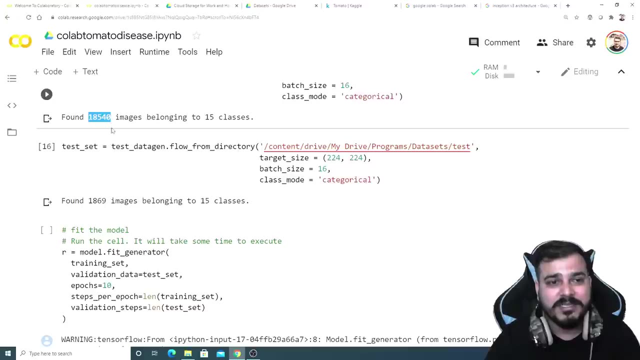 i think the ram- uh, it is less over here when compared to the ram that i had in my workstation. it was somewhere around 16 gb, so i'll also make this as 60, okay, but remaining all things are good to go. okay, i'll be executing this now. you can see that they are somewhere around 18 540 images and 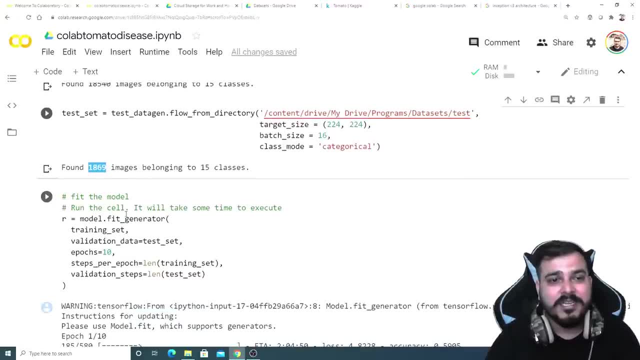 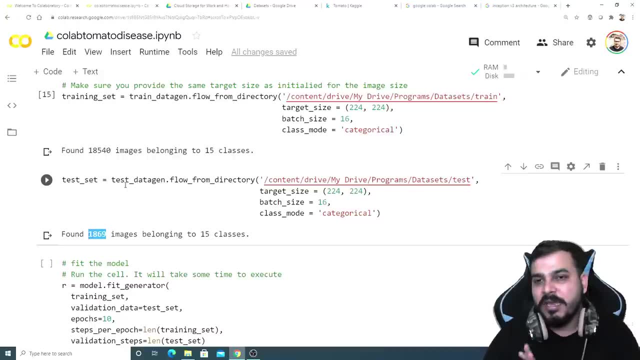 they are somewhere around 18, 69 images in the test set, then uh, probably this will take time. i'm not saying that this will take two to three days, but at least half to one hour it will take. uh, in my workstation this whole problem took me somewhere around 25 minutes uh for doing 10 epochs. 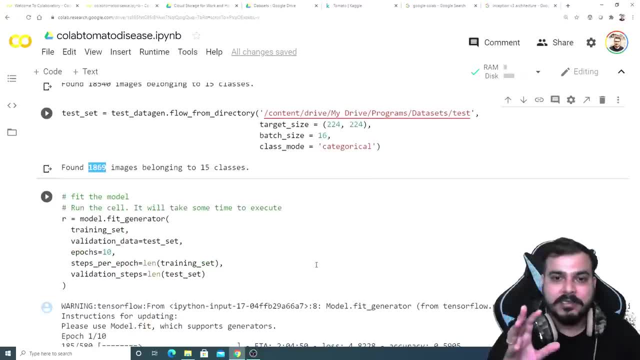 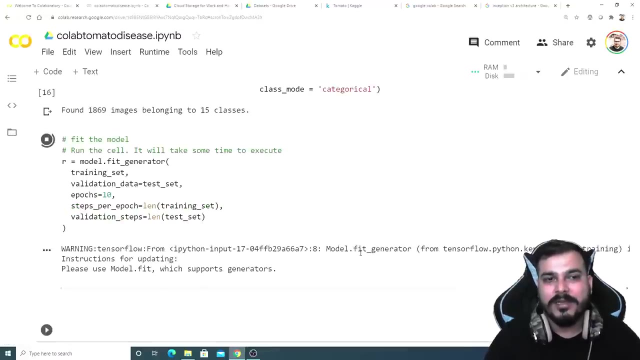 so, uh, imagine, with respect to that case, in my workstation i have 64 gb ram, i have titan rtx, which is 24 gb of vram, and uh all the processing speed is superb over here. so let's see how much time this will take. uh, just by understanding one epoch, i think you'll be able to find it out. yes, 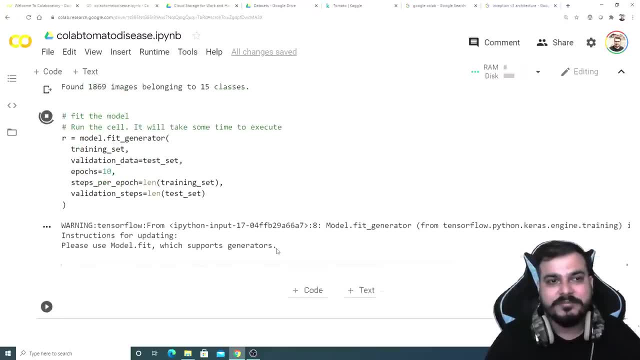 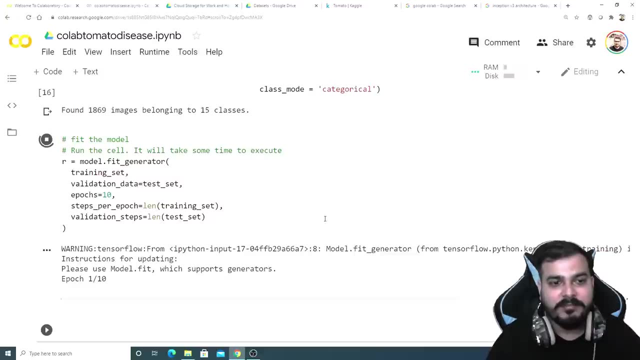 so instruction for updating the training has started. okay, the training has started. the epoch first has actually started. you can see that i've given uh epochs as 10, just to give you an idea about it. okay, so now you can train your model. this model training will happen and further code i have. 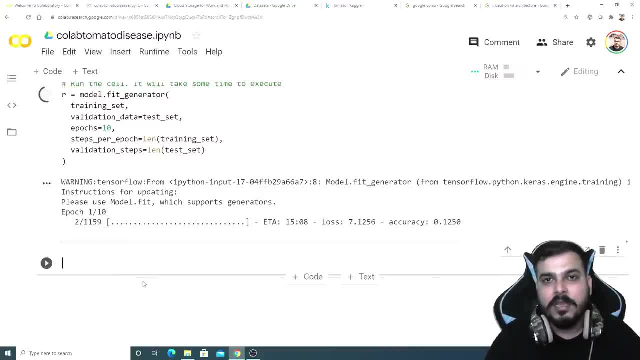 to still write it down. the further code will basically be to check, uh, how is the, how is the training accuracy and validation accuracy, um, by seeing a graph, and then, uh, probably we can do the actual. uh, i think, uh, this all kind of explanation i've done in my live project playlist where i've 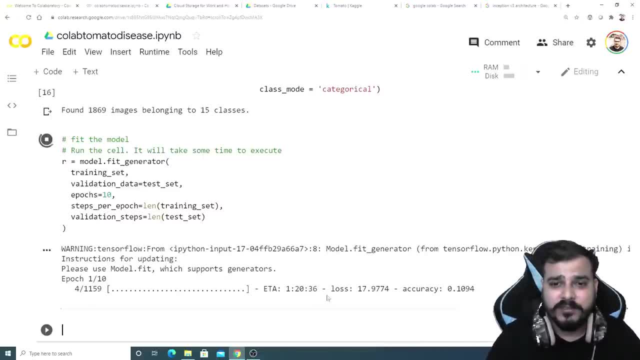 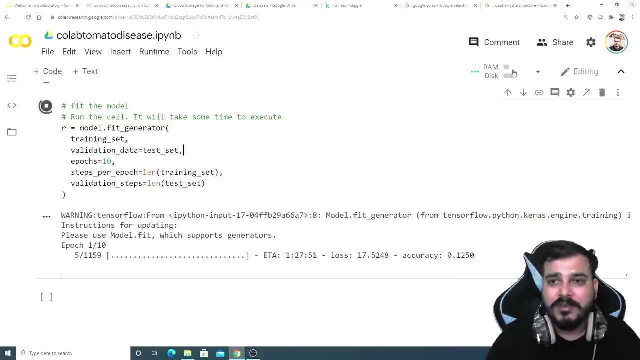 discussed about, uh, deep learning projects itself. so this will take some time. uh, the estimated time is taking somewhere around one hour 27 minutes. now you can see that the the ram size will increase or not, because the bass size i've taken at 16 loss is 16.46. accuracy is 1.1250. let's see how much time 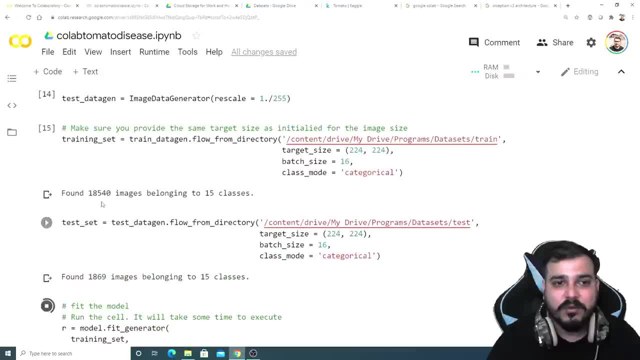 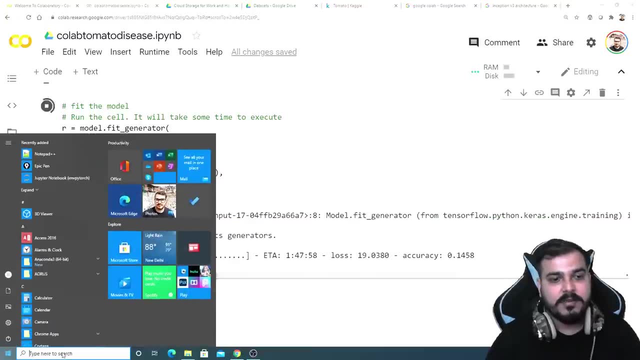 as a batch size, why i'm getting one. one, five, nine, that is basically the whole number of images, this 18, 5, 4, 0 divided by 1, 6, what it is? i think it is this much only. let me see. i'll just open the. 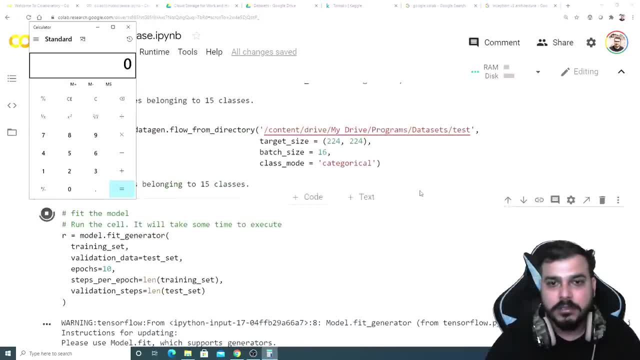 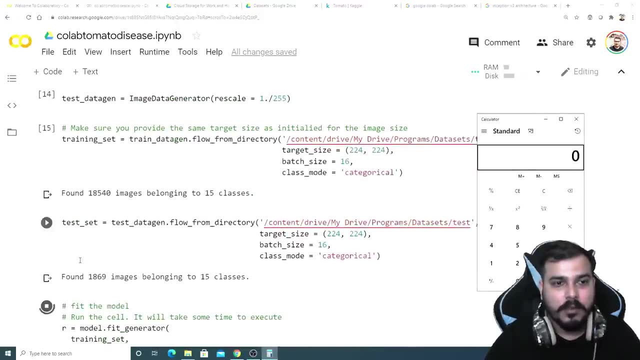 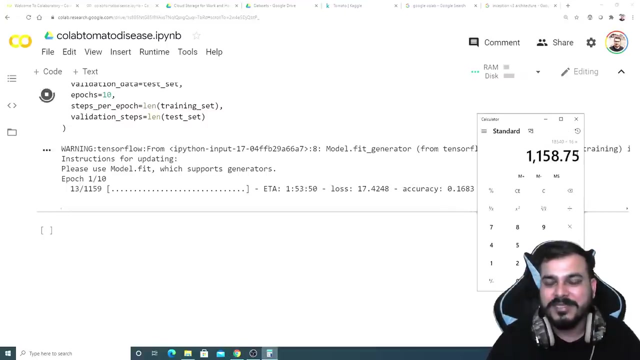 calculator. so what are the total images? that we had 185, 185, 4, 0 divided by 16: 1, 1, 5, 8, right? so here you can see that 1 1, 5, 9 is basically taken up, because i think we got 1 1, 5, 8.75. this is basically the floor part, and here you'll be. 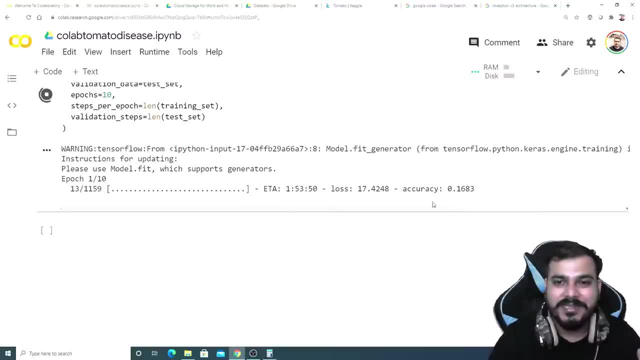 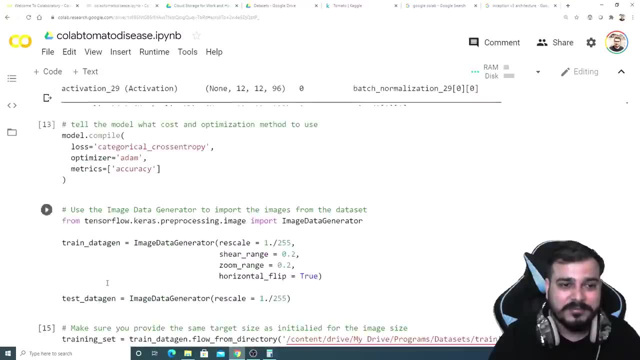 seeing that after some time, the loss will be decreasing, the accuracy will be increasing and, yes, it will take time because it has more than 8000. 18000 images, guys, so 18000. but just try it by yourself. you have just have to be patient for around one hour just. 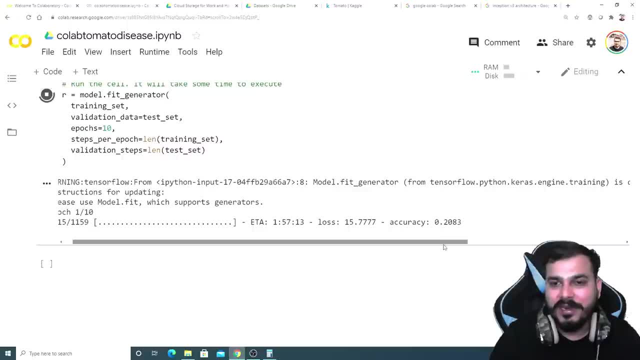 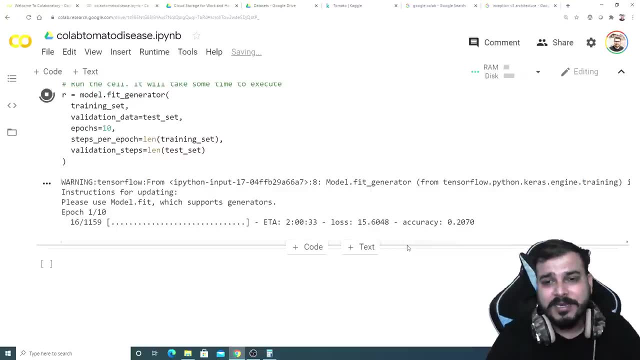 keep it like that and this particular accuracy will be running okay. so let's see how much time it may take and, yes, you can try it out. so but again, understand, the overall idea was to show you how you can train deep learning model images and all because in the upcoming 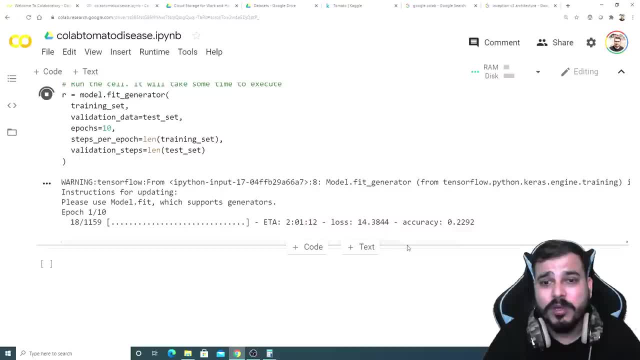 videos. i'll be showing you bert, i'll be showing you transformers, i'll be showing you advanced nlp techniques and definitely, since you don't have a workstation, google collab will be the best option for us, so that you'll also be able to learn efficiently for but for the people who have workstation. 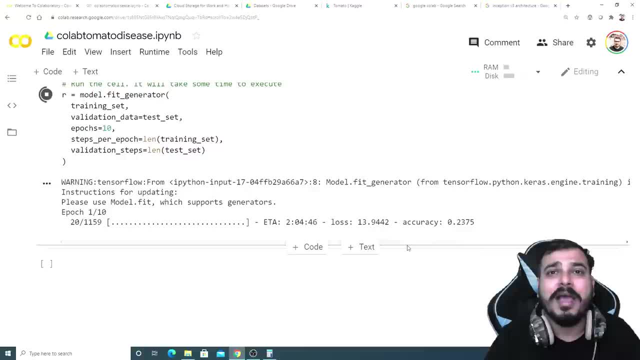 i think you can just do the installation automatically. all the execution will happen and probably, guys, in the future i'll also be coming. i'm also making a partition of linux system in my, in my workstation so that you get an idea of how to train models in linux, how to work. 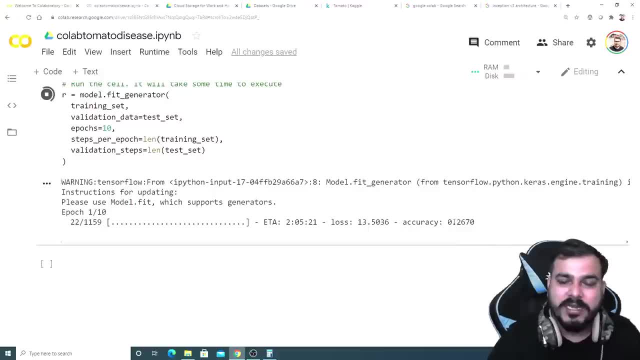 in linux and all so here you can see that initially it was 0.18 accuracy. now it is increasing to 0.26, at least for one epoch. i'll show you and we'll see the accuracy. let me just fast forward this thing. how do i fast forward? so let this run, okay, but it'll be pretty much. 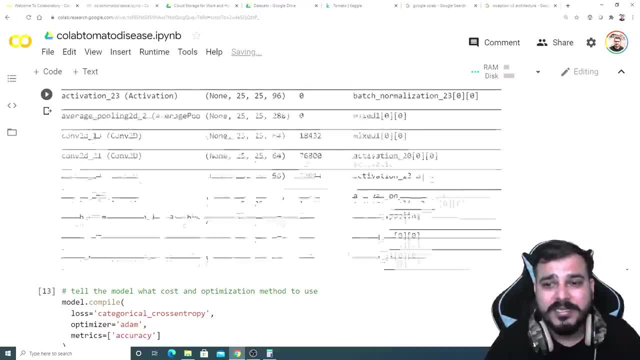 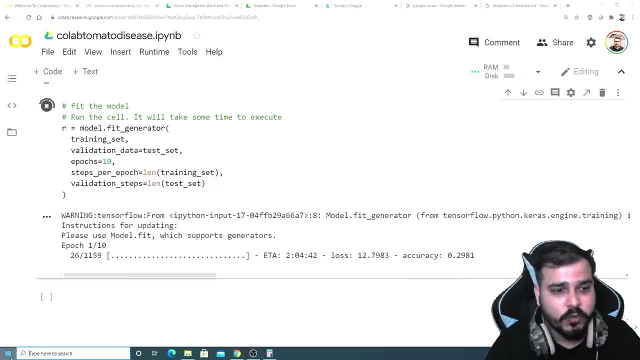 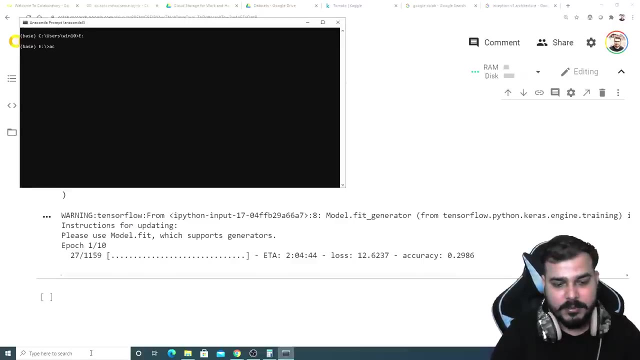 amazing. so this is what you can do, guys, with respect to all the data sets. just let me know after one epoch, because i have already tried it out in my local system. let me just show my local system. uh, uh, uh, pop up, Activate My e and v1. oops, my e and v, and I'm going to open the. 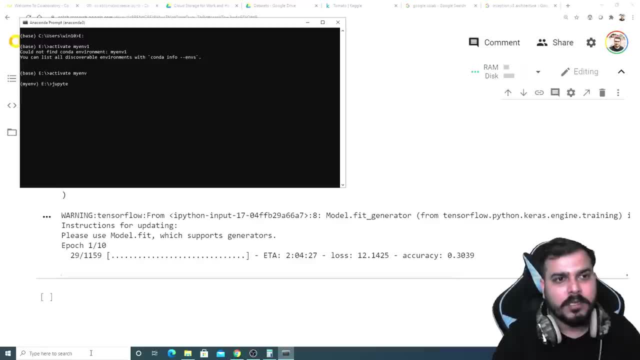 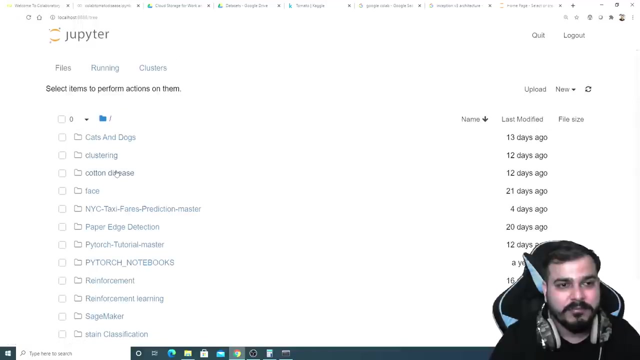 jupiter. Okay, let me just show CD deep learning. okay, then I think it is Jupiter notebook. I'll open the Jupiter notebook over here. I had created an environment, separate environment, for this, so This was NYC, which I was doing for the members, And it is. this was the tomato disease. Yes, plant villages. 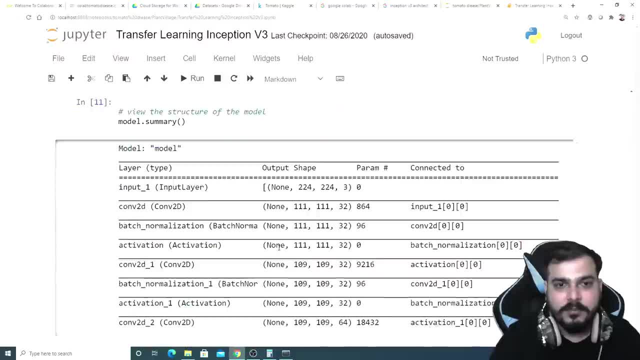 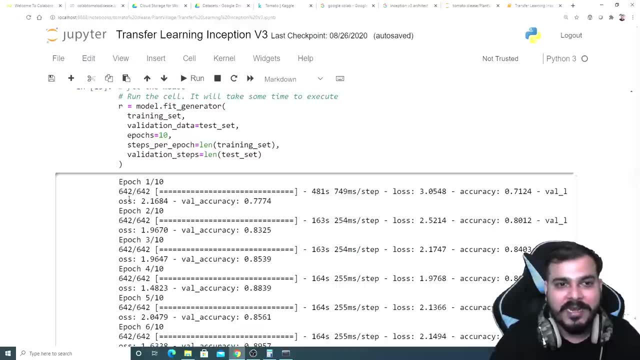 So here, if you see, with respect to inception v3, when I did the training in my local, You know it was taking every. every epoch was somewhere taking around, and here I had also Increased the bass size. I think I made the bass cries to 32.. Okay, so here it was saying that. 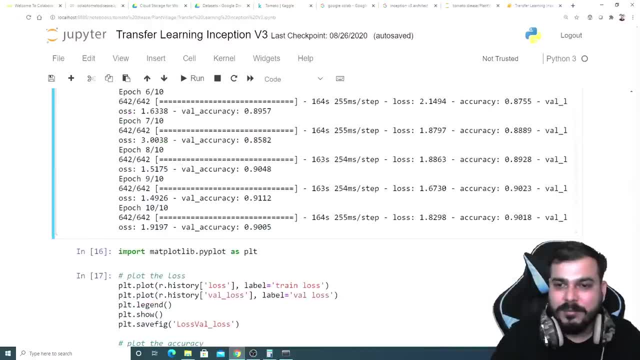 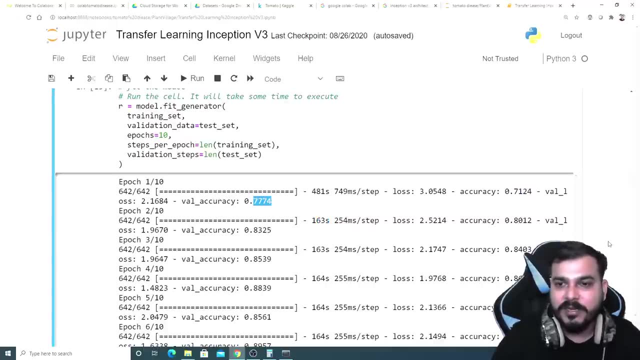 It was taking for 81 seconds, 163 seconds every park. but the final accuracy just after the first epoch only I was able to get somewhere on 71 and the validation accuracy was somewhere on 77%. ok, but here at the end of the day you'll be able to see that our training accuracy was. 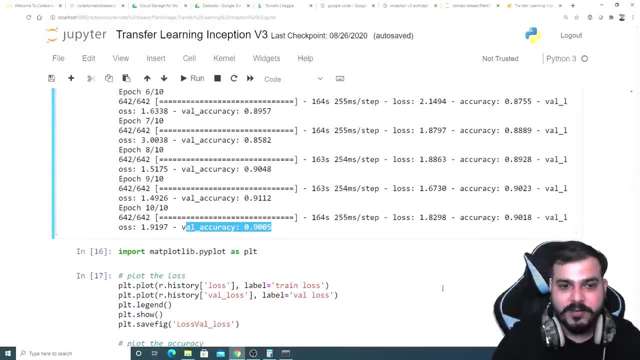 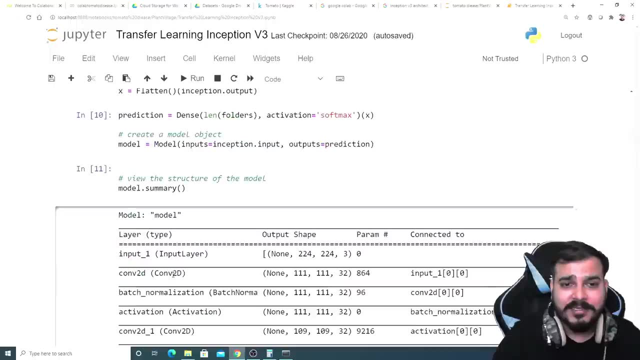 0.9. 0 and your validation accuracy was 0.9.. 0.05. so I will be putting down this whole. I'll be giving this whole code to you all. what you have to do Is that just change this particular path based. 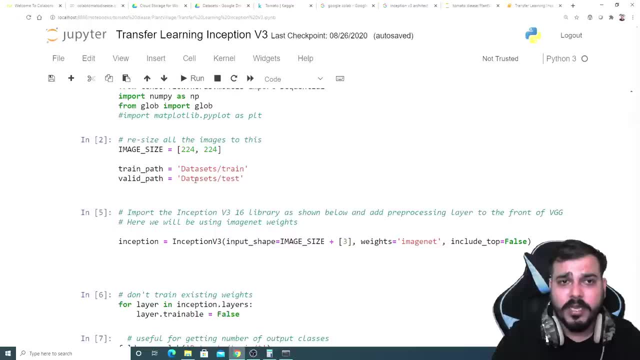 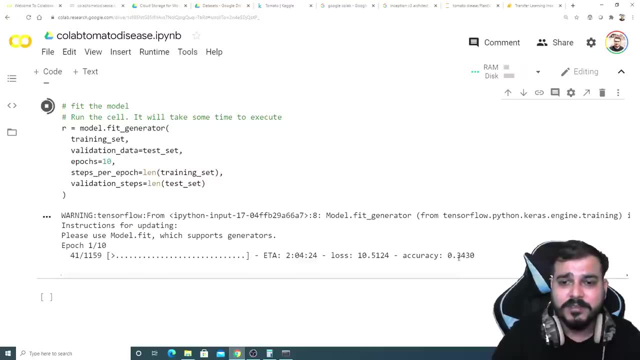 based on the path of a google drive, wherever you are uploading. okay, till then, i think this will take some time. now you can see that my loss has decreased from 16 to 10 and my accuracy is also increasing, but, in short, it will be looking something like this: only make sure that when 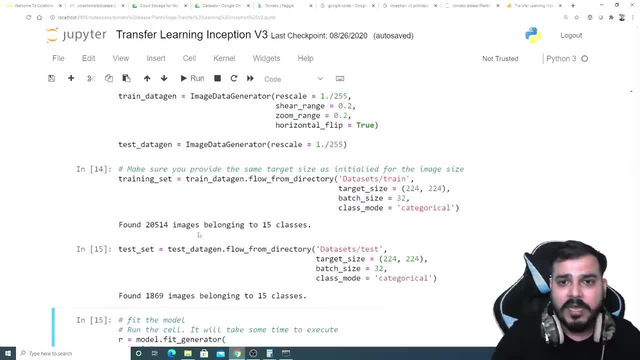 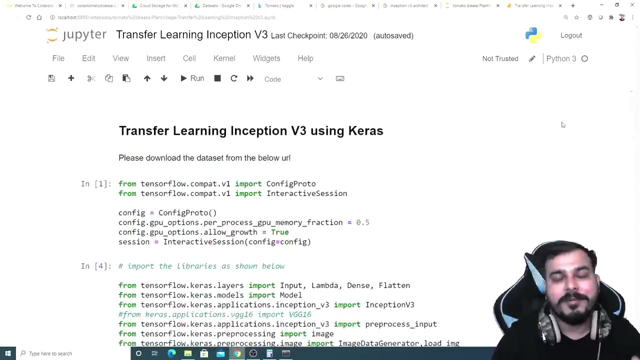 you are training in the google collab, make sure that you make this batch size as 16. that is it okay, and just try to execute this. so i hope you understood this. i hope you found this video very, very much useful. uh, please do subscribe the channel. if you haven't already subscribed, i'll 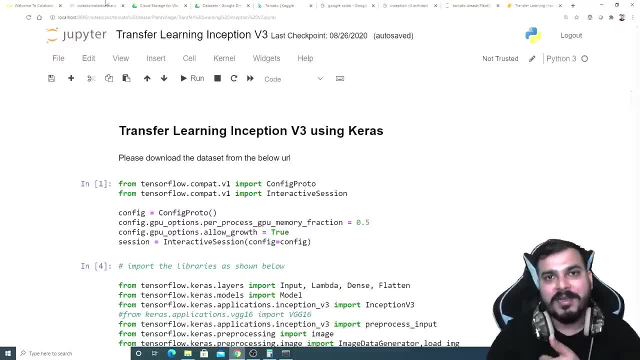 see you in the next video. have a great day, thank you and all bye, bye. cheers to google collab. cheers to google. thank you. 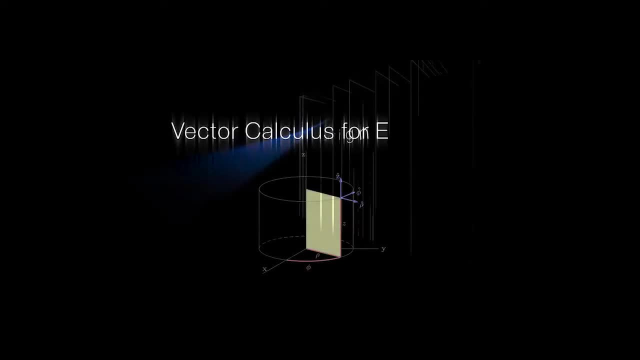 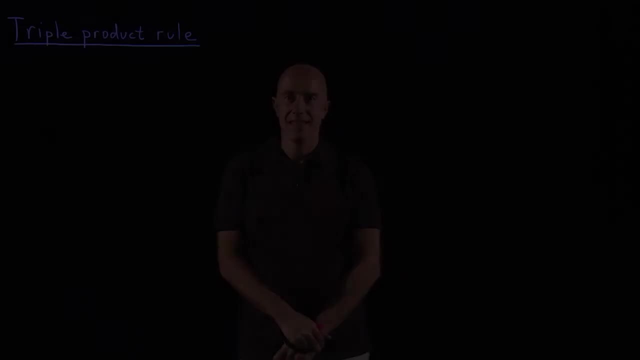 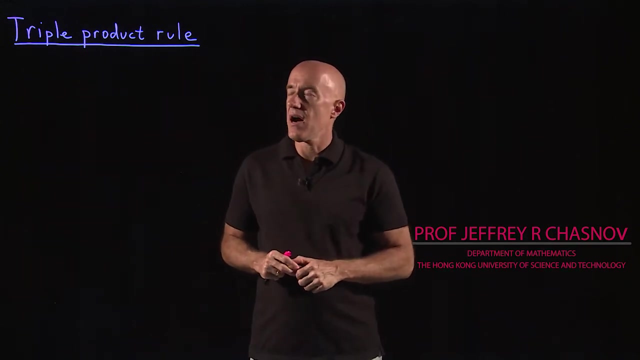 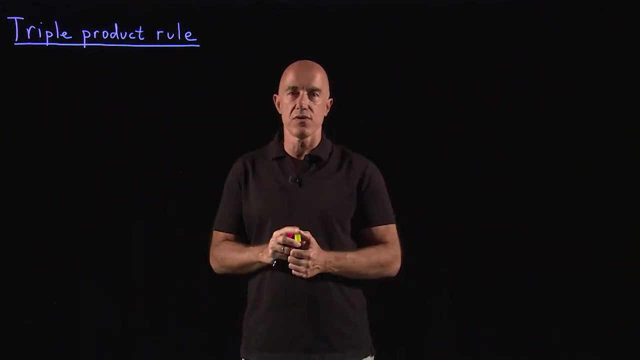 So we learned about the chain rule and when I derived the chain rule we did some differentials. There's another use of differentials to derive the triple product rule. The triple product rule comes up a lot in chemistry when you discuss thermodynamic quantities. So someone